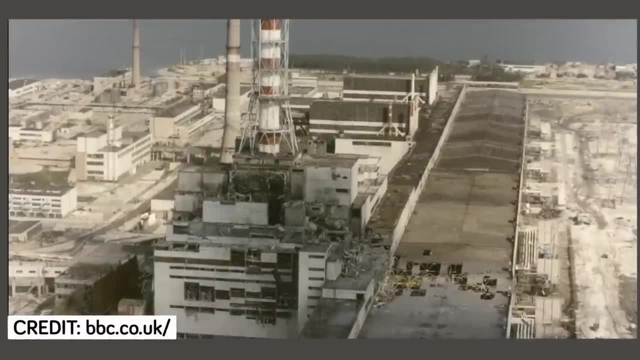 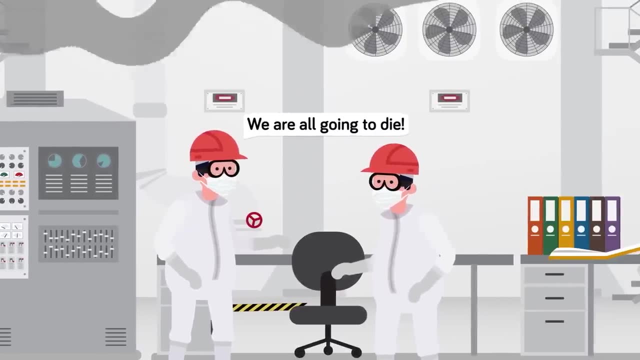 will not want to admit What the capitalists can do. they can do just as well, Or so they think. One thing you don't want at a nuclear power station is a total shutdown. If that happens, things can heat up And if an explosion follows, what you have is a massive leakage of deadly 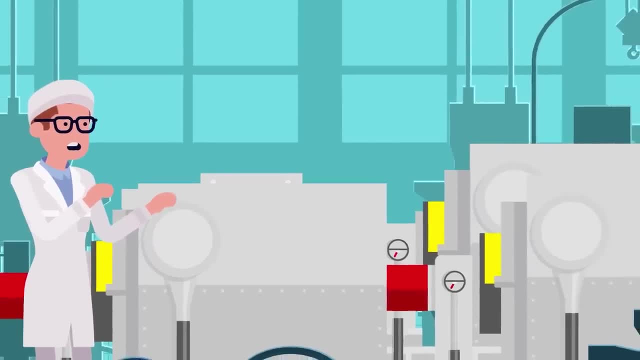 radiation. So every reactor at Chernobyl has three backup diesel generators that will kick in if power is suddenly lost. If the power is suddenly lost, the reactor will be shut down. If the power is suddenly lost, the reactor will be shut down. If the power is suddenly lost, the reactor will be. 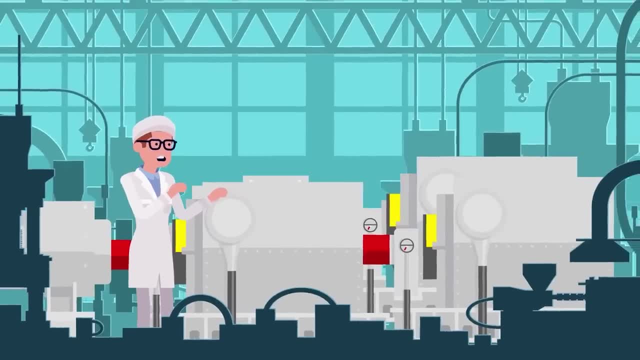 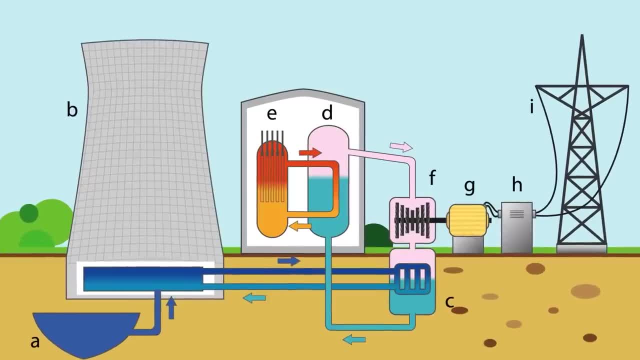 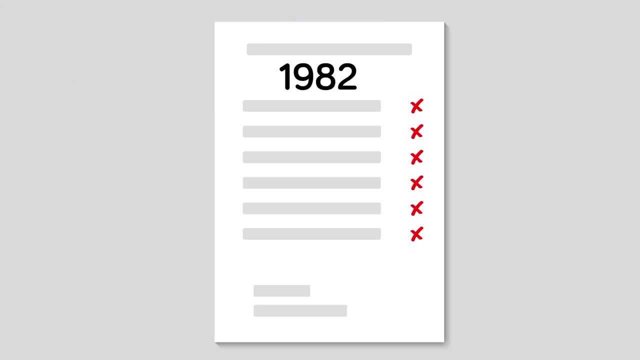 theory is that the slowing turbines after being turned off will create enough electrical power to keep the pumps running during that gap before the generators are running at capacity. To know if this works, they need to do some tests. The first came in 1982,. 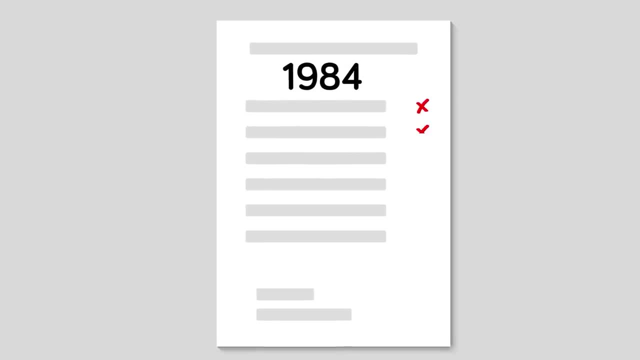 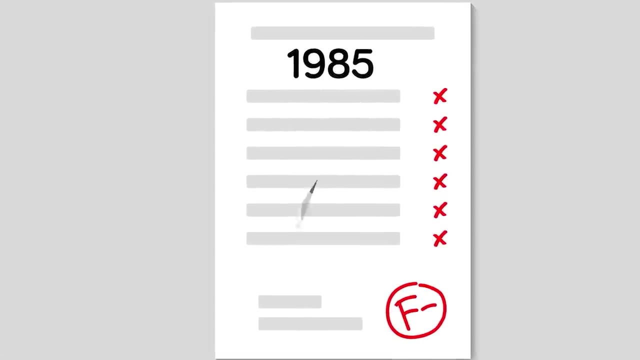 and it wasn't successful. They tried again in 1984, and again the results were not good. Then they tried in 1985, and yet again a message was sent back to Moscow saying things hadn't gone as planned. This was not what the bigwigs wanted to hear, and they made that known. 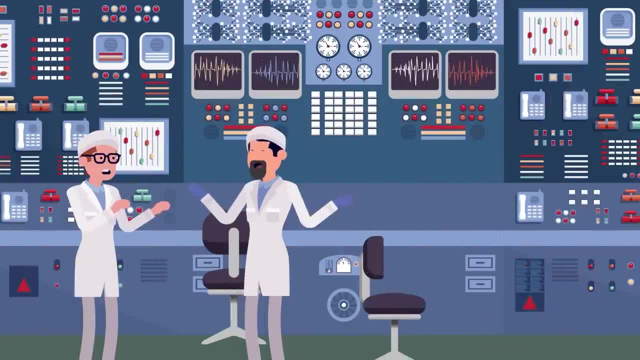 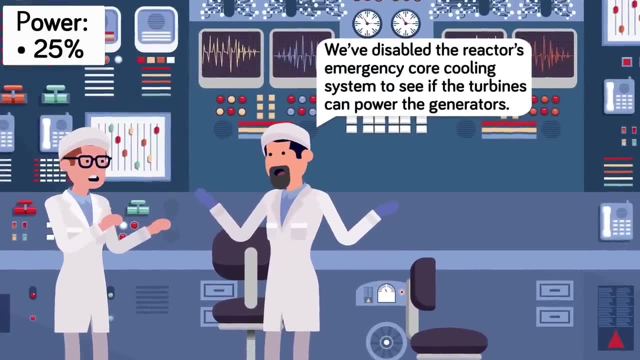 The pressure was on. Excuse the pun. The reactor had already been slowed down to run at about 25% of its normal power. Importantly, the reactor's emergency core cooling system had been disabled, so it didn't get in the way of seeing if the turbines can power the generators. More importantly, 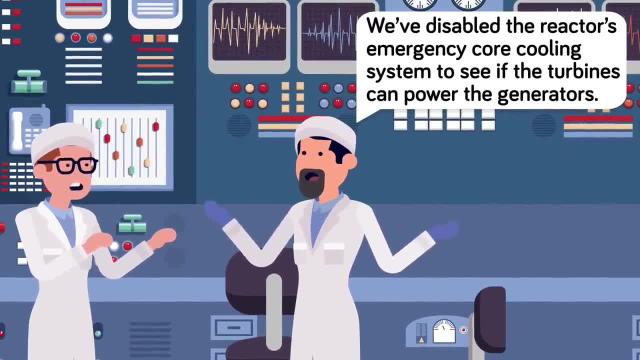 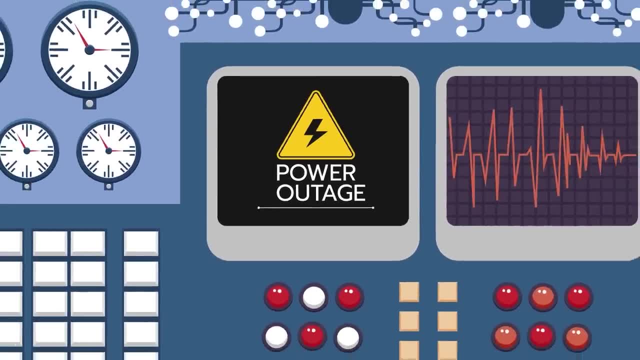 some of the night shift workers that have arrived haven't been properly briefed about the test. The reason is the test should have happened on the day shift, but there was a power outage earlier in the day at a coal plant, so Chernobyl had to keep running at full power to give people their 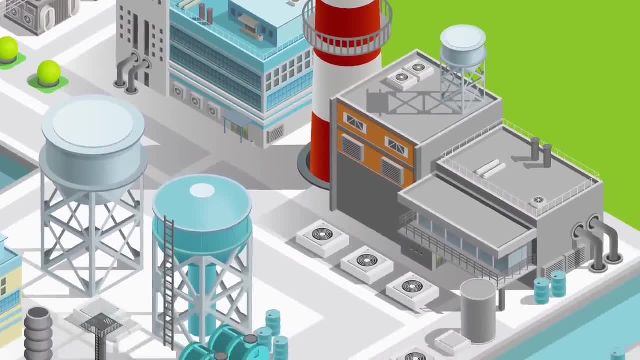 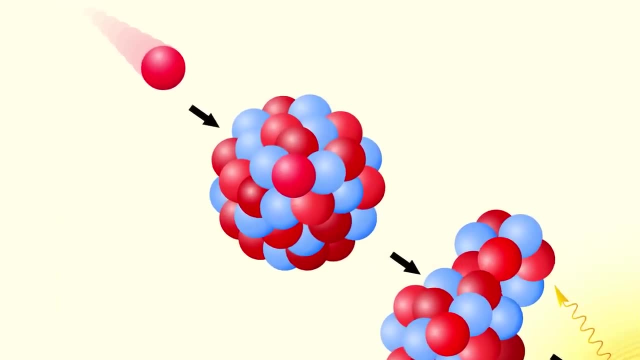 electricity. To fully appreciate this story, you need to know how we get the electricity from a nuclear power plant. so here we'll give you the very basics in layman terms. Inside the reactor, neutrons split uranium atoms and that makes more neutrons. They split more atoms. 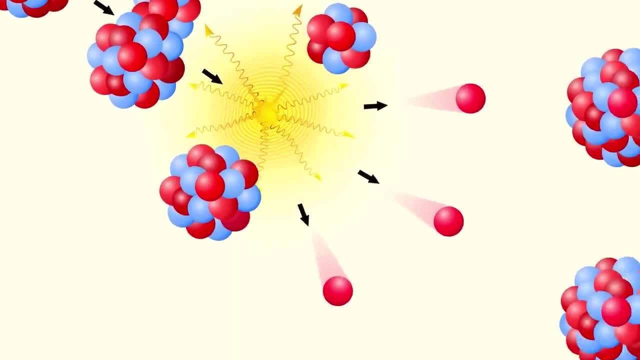 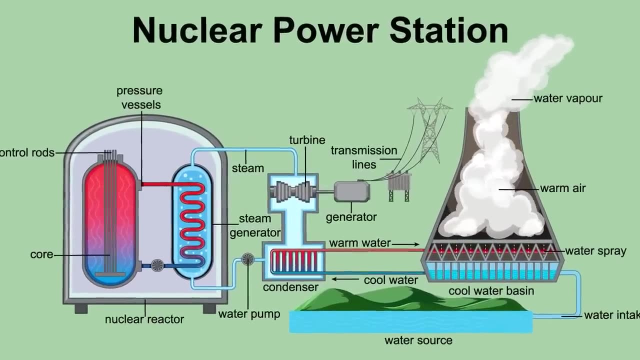 and we have more neutrons and so on and so on. This is a chain reaction and it produces a crap load of heat. You harness the heat and make it turn water into steam, and the steam runs those turbines that we are working with. This is a chain reaction and it produces a crap load of heat. You 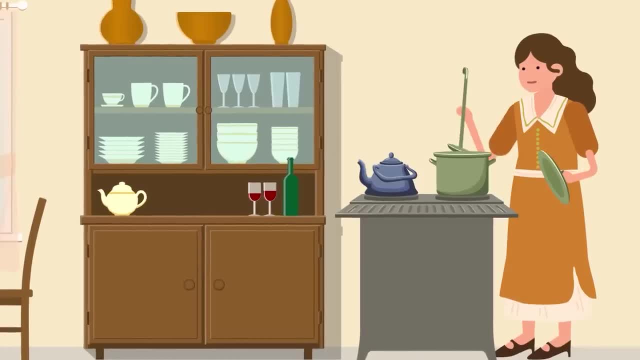 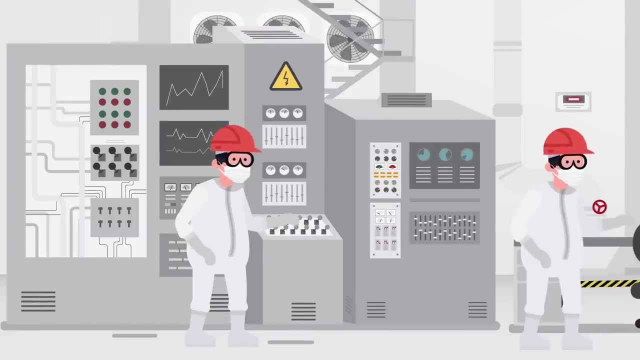 harness the heat and make it turn water into steam, and the steam runs those turbines that we already talked about. As they move, all this energy becomes electricity that ensures people like Natasha can cook clean eat, see, watch TV and stay warm in winter. All that heat and energy. 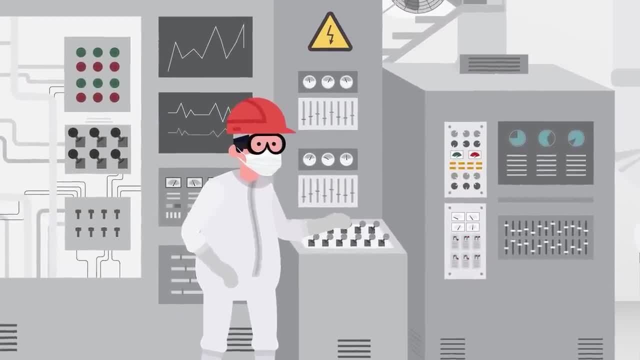 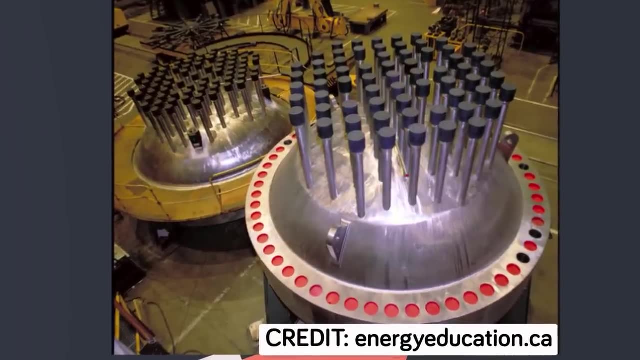 of course, can be a bit unstable, so you have to control mechanisms to make sure there isn't an overload. If not, the chain reactions would just keep going and become highly dangerous. Control rods are the things used to slow down the chain reactions. These are a bunch of rods that. 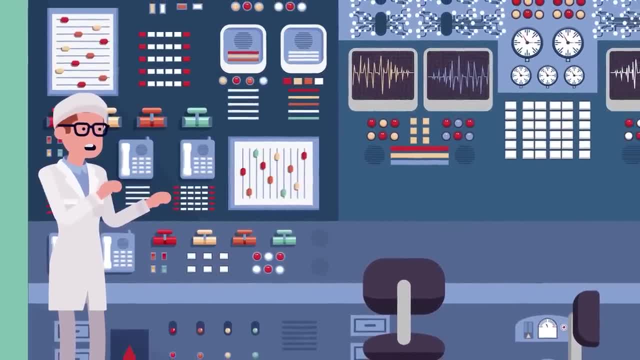 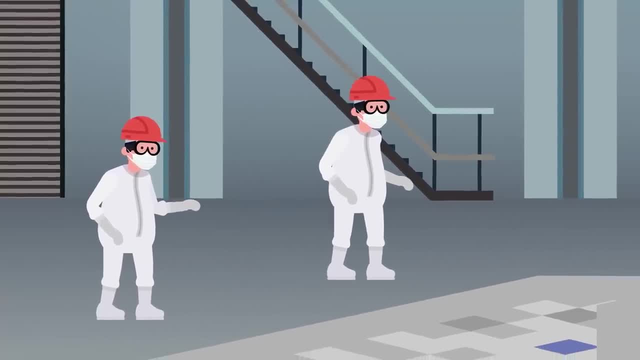 can be inserted into the reactor in different numbers or in different lengths, allowing the nuclear technicians to control the rate of the nuclear chain reaction. They're made out of special materials that can absorb neutrons, so if all does suddenly go to hell, you will at least. 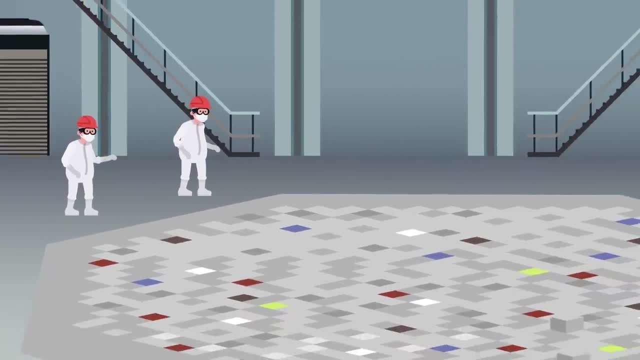 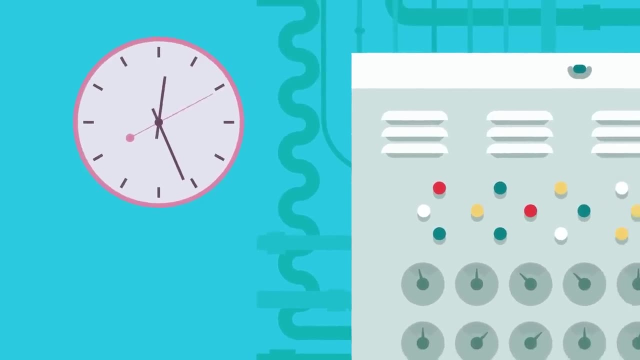 hope these rods can come and save the day. No one at Chernobyl doubts their safety, or at least the less experienced operators don't. Hour 1: Now you know the night shift isn't properly prepared for the test and it might be their fault that the power out of the plant falls too much at 28 minutes past. 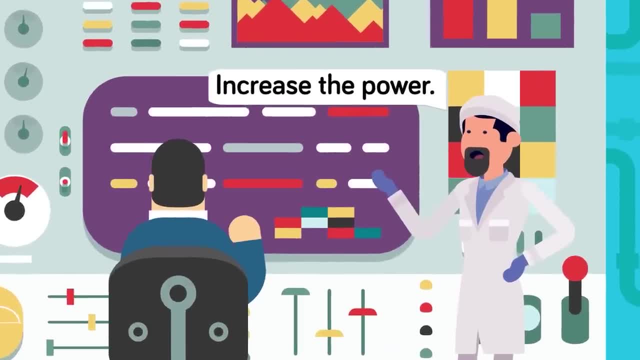 midnight on April 26th. They try to increase power, but something's wrong. They're trying to slow down the chain reactions. They've never seen this before. This is partly because there's been a buildup of xenon during the test. 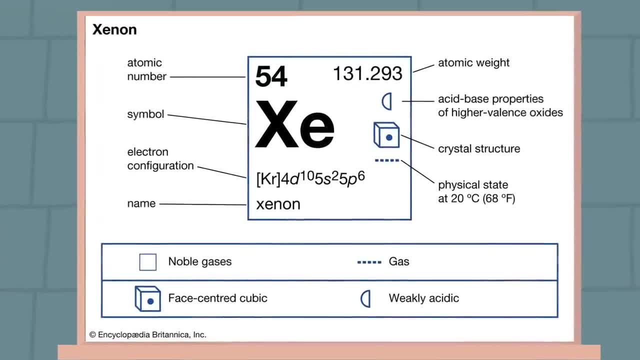 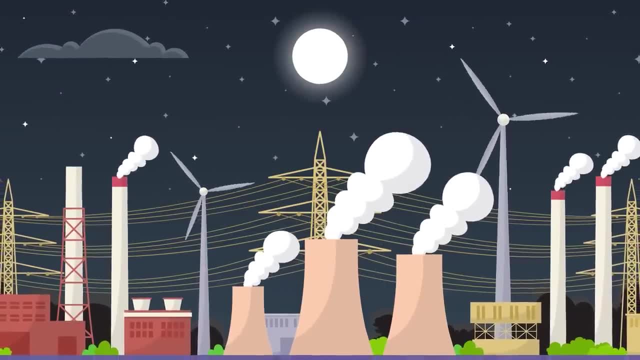 You don't need to know what xenon is and, to be frank, it's too complicated to fully explain- but when there's a buildup of the stuff it can cause xenon poisoning. Xenon would usually burn away when the reactor is at full power, but the slowdown has caused a buildup. 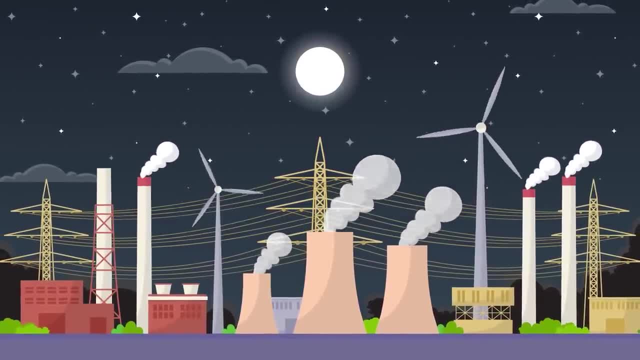 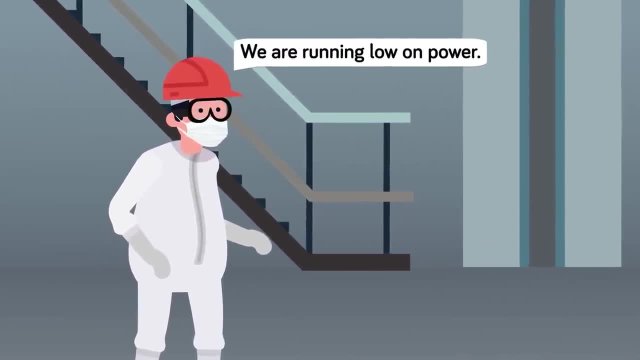 and the buildup has caused a further slowdown. This is not good. It's because of this overabundance of xenon that even when the guys take most of the control rods out- 200 from 206, they still can't get enough power. As you know, by taking out the rods they should get more power, since the nuclear 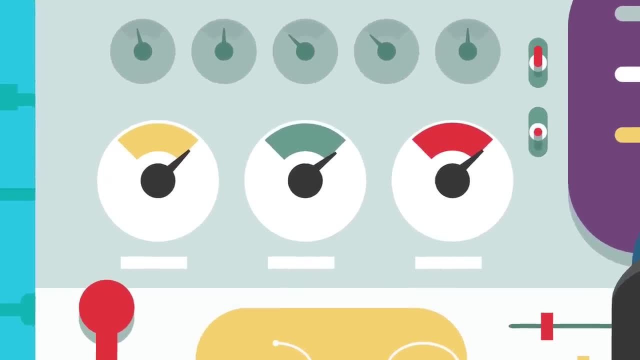 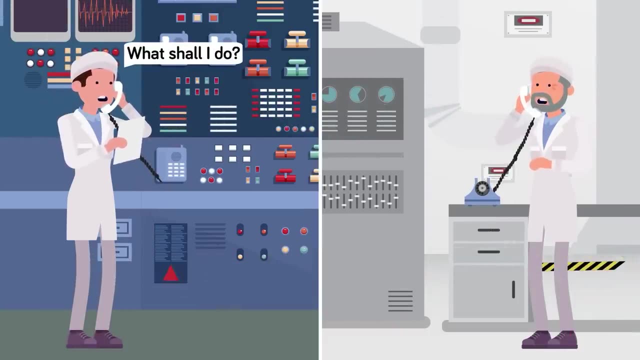 reaction isn't hampered. Doing this, though, can be pretty dangerous. In fact, they shouldn't be doing this in the first place. A young operator gets on the phone and asks: what shall I do? In the program, there are instructions of what to do. 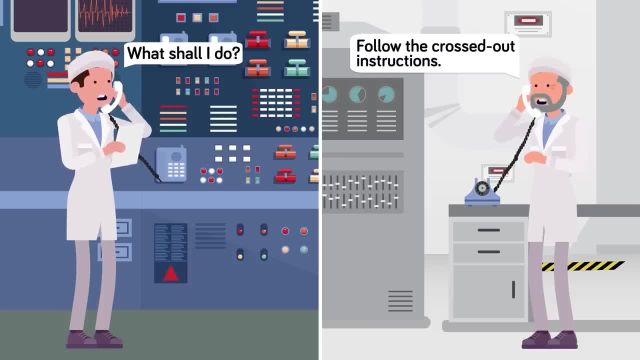 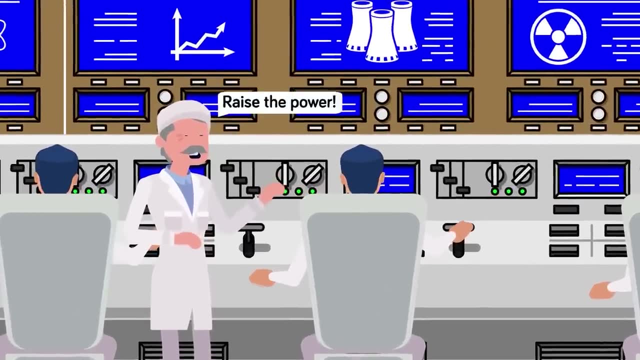 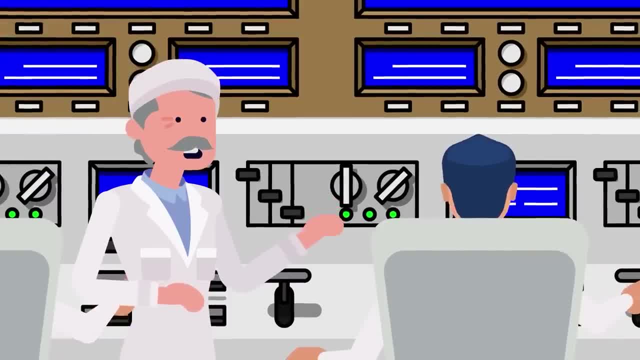 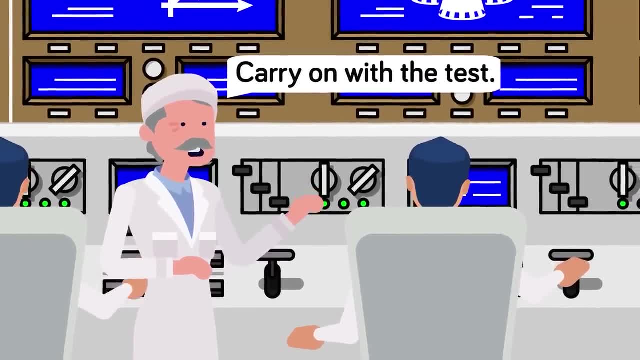 but he was. don't forget his name. The reactor is certainly running at less power than is safe for a test, but they carry on anyway on the orders of Dyatlov. He doesn't want a black mark against his name in the form of another failed test. 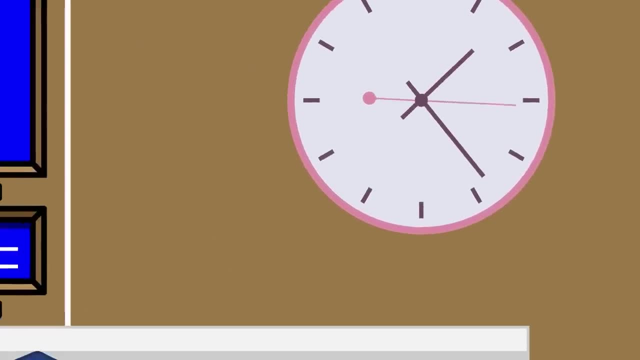 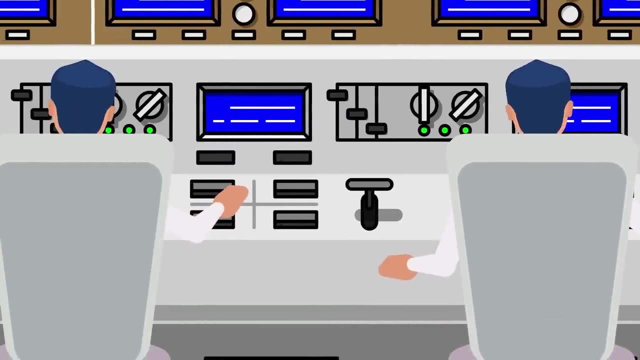 At 1.24 and 4 seconds the test really starts, meaning they're going to simulate a power outage and, as we have explained, see if the slowing turbines can power the coolant pumps before the generators can turn on. This is when all hell breaks loose. What happens is a sudden and massive increase in power. It is 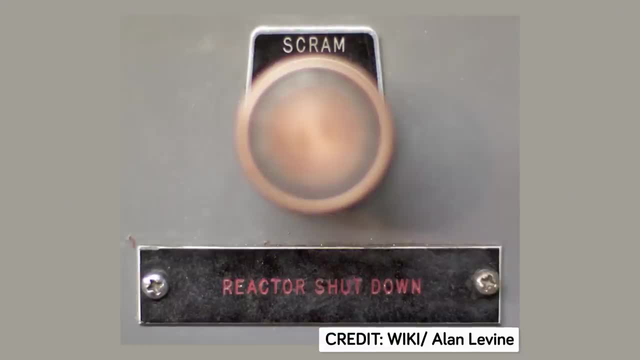 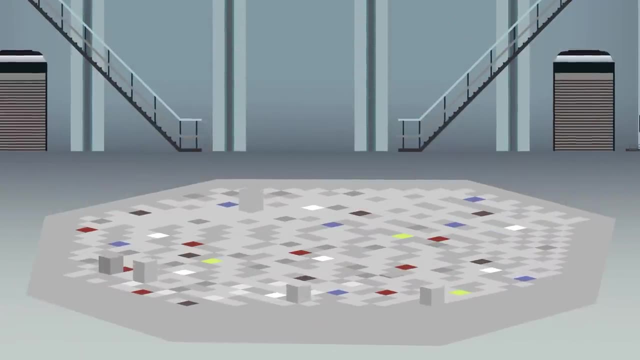 dangerously high, and this is now very serious, So serious that someone hits the scram button At Chernobyl. this was the AZ-5 button. It's an emergency off switch which makes all the control rods drop down to stop the nuclear reactions. This is a big mistake, and one. 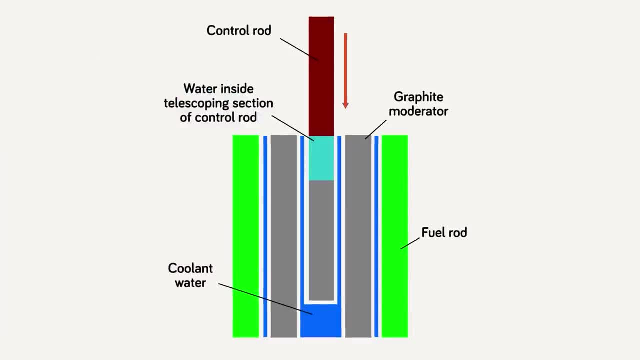 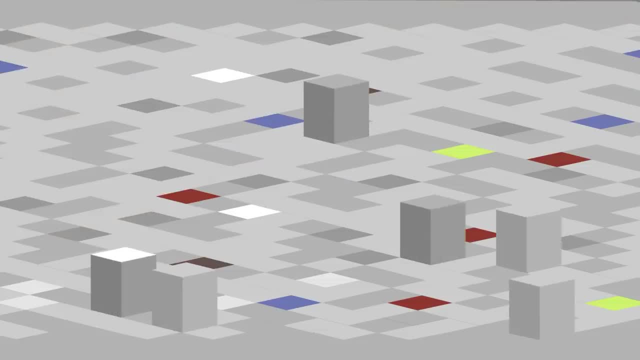 which exposes a few of the design flaws at Chernobyl. The rods have a graphite tip which, in short, actually increases the reaction rate, not the opposite, as wanted. The boron in the rods reduces reactivity, but not the tips, As so many rods hit the reactor. 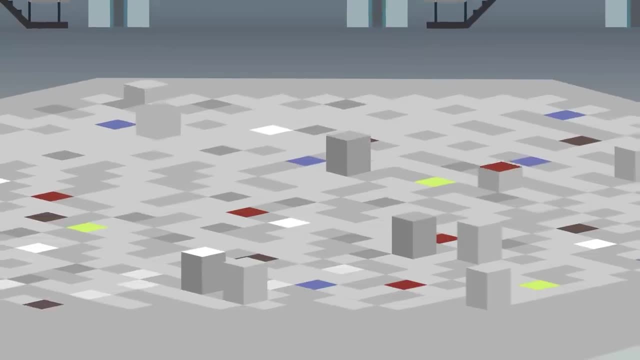 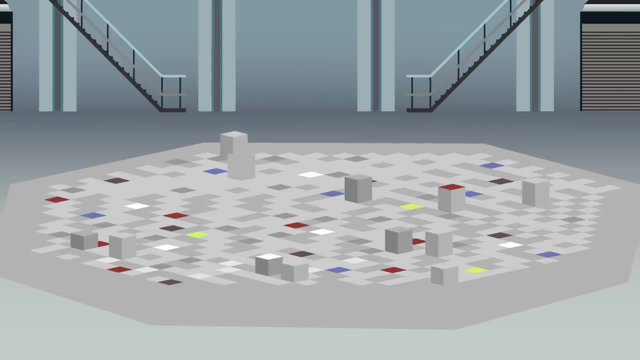 at the same time, there is a huge surge in reactivity. The operators don't know what they've done. The graphite tips are fixed in position and the heat creates a massive amount of hot steam- In effect, a bomb. The operators are not aware of this, or they wouldn't have. 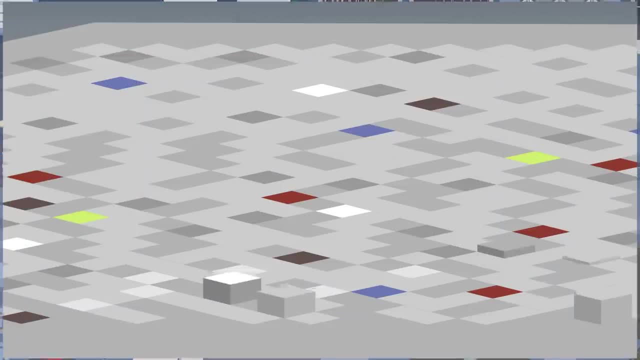 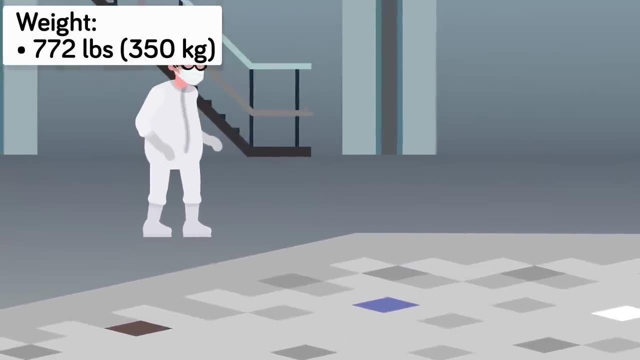 dropped the rods into the reactor, already surging with power. The man in the reactor hall watches as this happens And is shocked to see those 200 rods and their caps, each weighing 772 pounds, jumping up and down with the reactor lid. It's as if they're being pushed by the power of God. 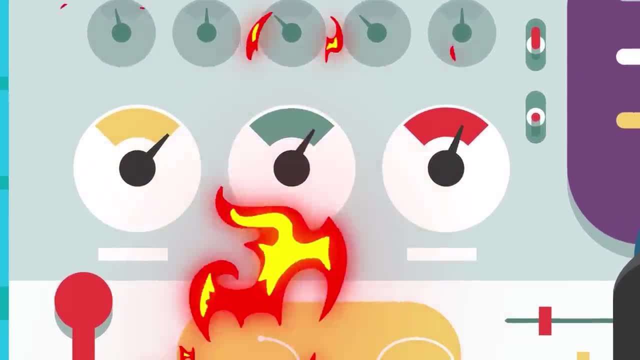 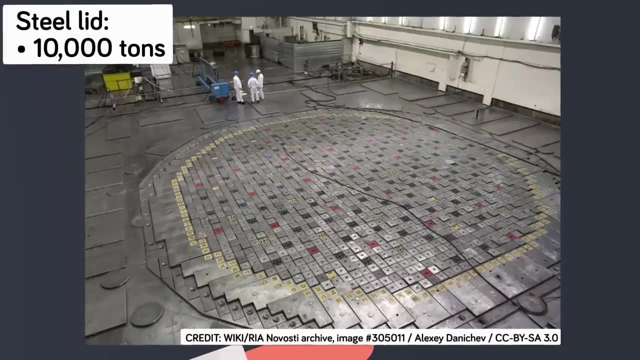 The output of the reactor is now at 10 times the power it should be. and that's it Bang. The bomb goes off. The world will never be the same again after this moment. The explosion causes the reactor's steel lid weighing about 10,000 tons or 2,000 medium-sized. 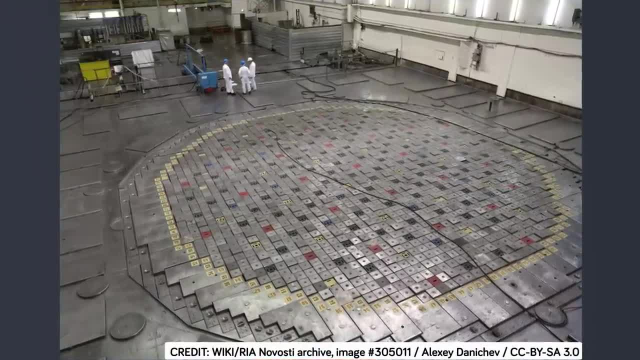 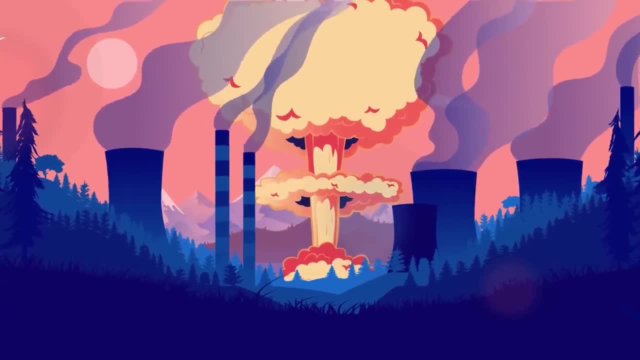 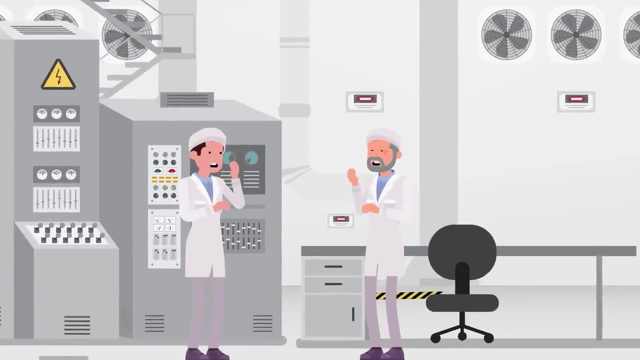 male African elephants to fly off and go straight through the roof. Shortly after there's another big explosion, likely down to a build-up of hydrogen from zirconium steel reactions. Bits of radioactive material and fuel are sent everywhere, Fires rage and the core is exposed to the world. Right now it's not obvious to most of the men in the 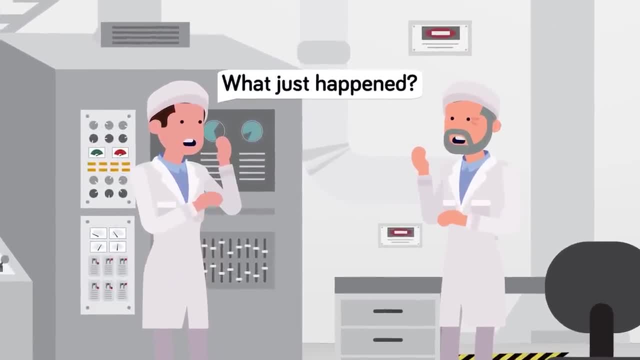 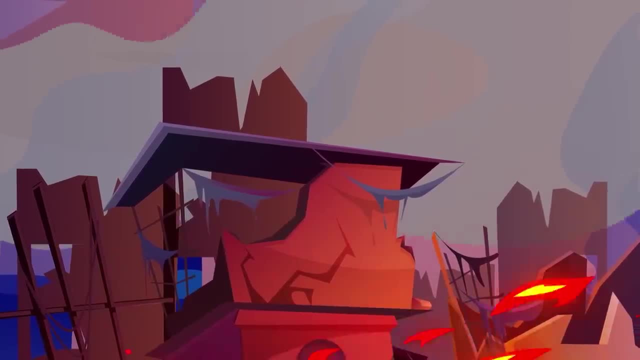 plant. what's happening? They all think the reactor is still intact, only because reactors normally don't just blow up. The roof is destroyed, The floor is in pieces, Radioactive materials are lying about everywhere, The air is filled with clouds of dust, Pieces of radioactive graphite. 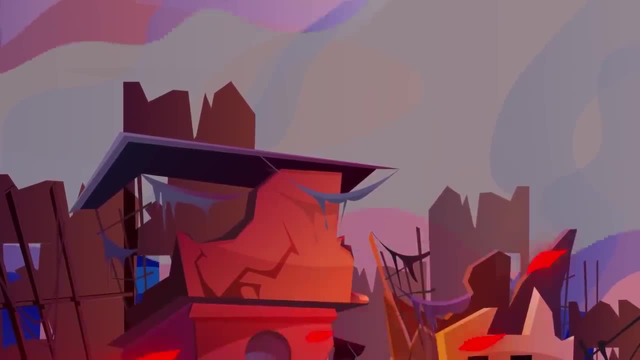 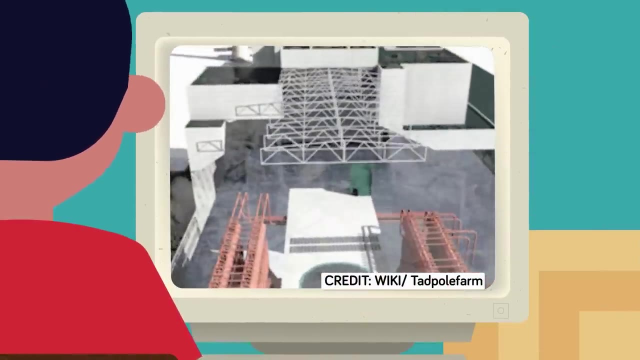 are flung great distances and radiation is now spilling into the atmosphere. To say this is bad would be putting it lightly. Soon a few men will know this, but one that knows it best will be too dead to tell the story. 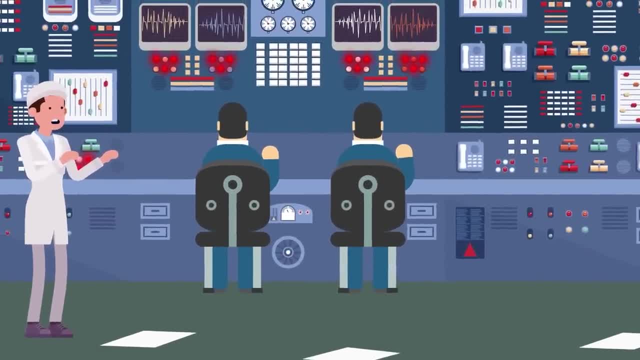 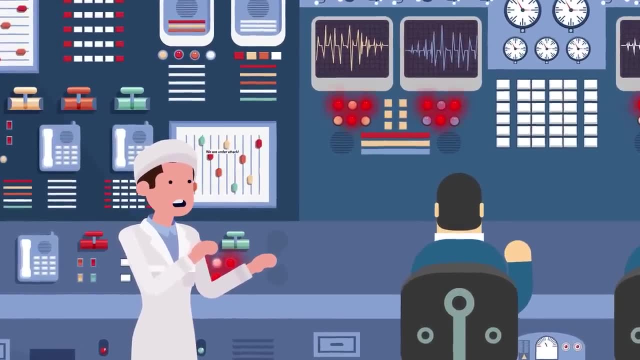 Right now, Alexander is in a state of shock. Just a moment ago he was in his office with some colleagues reading some documents, but now everything around them is shuddering on the brink of what feels like imminent collapse. His first thought is this: is war The USA has? 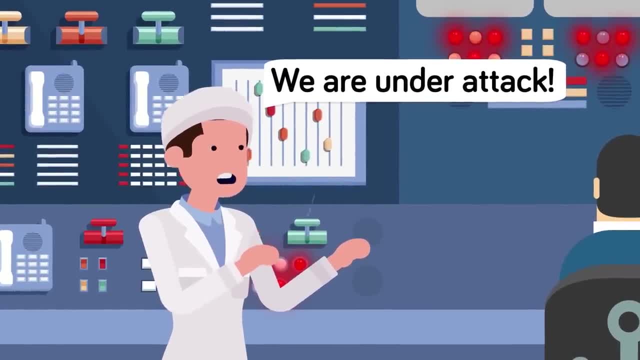 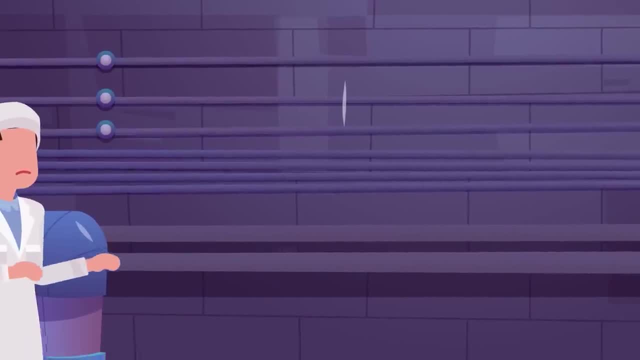 attacked us. He's not alone in thinking this. What else could have happened? The phone rings. It's the guys from Building Number 3. Bring some stretchers. they shout over the noise. Alexander takes off down some dark corridors in search of the men he knows are the closest to the explosion site. As he gets, 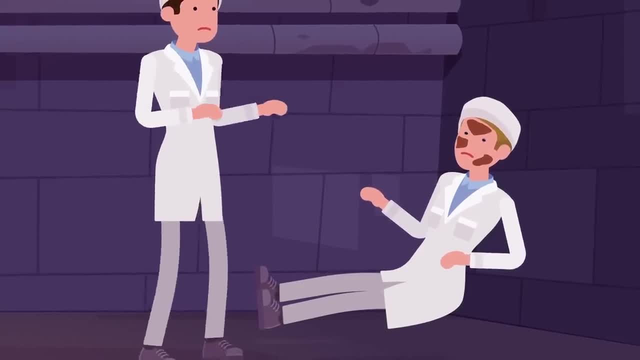 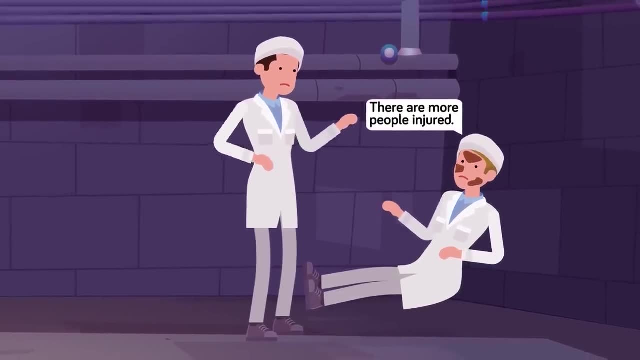 closer to a deafening hissing sound, he finds his buddy. His face is horribly disfigured, so much so that he knows only who it is. when he hears the sound of his voice. More people are injured. the guy tells Alexander. 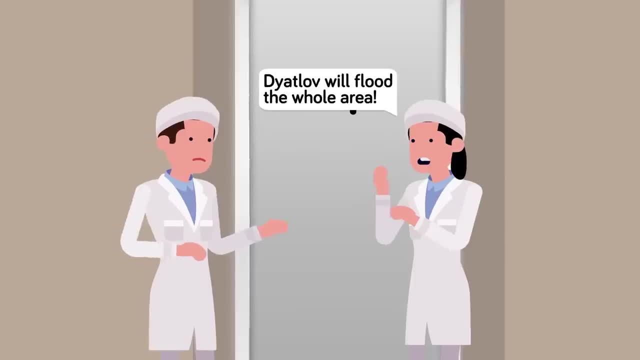 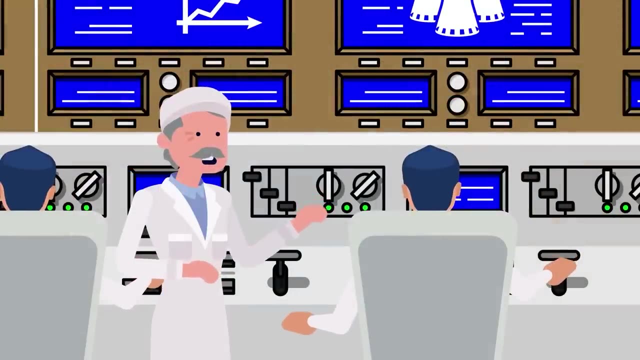 He then meets with Yuri Trigub, who's come from Control Room Number 4. He tells Alexander that Dyatlov has asked for the emergency high-pressure coolant water to flood the area. Dyatlov still doesn't know that the reactor has blown and he won't even believe it when he's told. 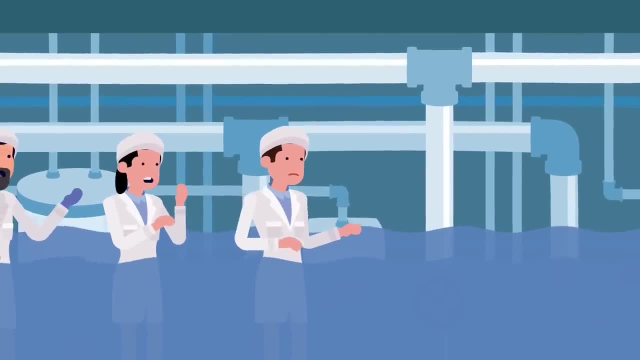 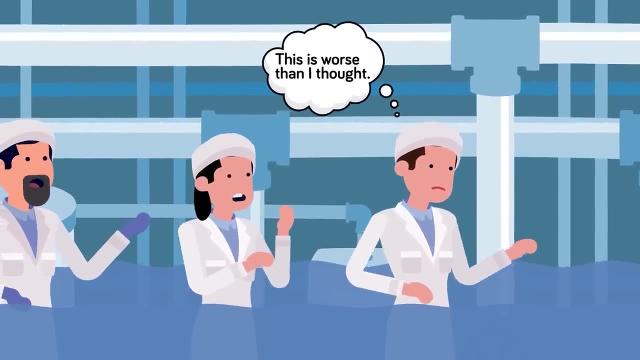 Now waist-deep in water. Alexander and a few other men try to get to the coolant taps, but through the door they see the giant water containers have been blown apart. All the men are terrified. This is worse than they thought. Alexander looks around at what's. 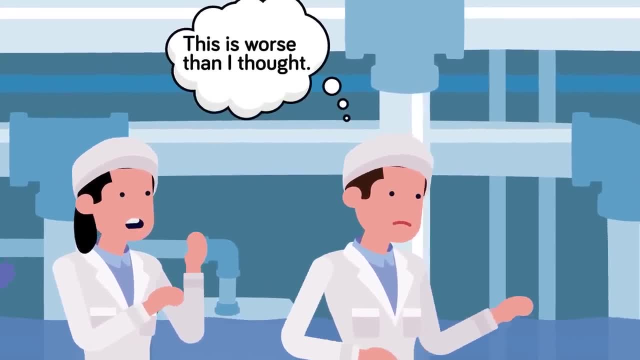 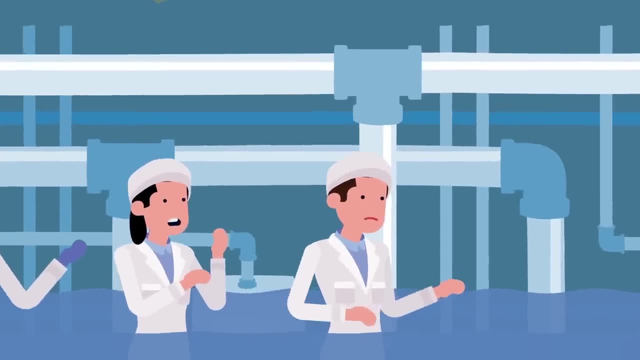 left of the room and sees his colleague Kodyemchuk on the floor, dead. He then looks up at the roof, or where the roof was, and he sees something magical: a great beam of light reaching to the heavens. It's magnificent and beautiful. He then looks up at the roof, or where the roof was. 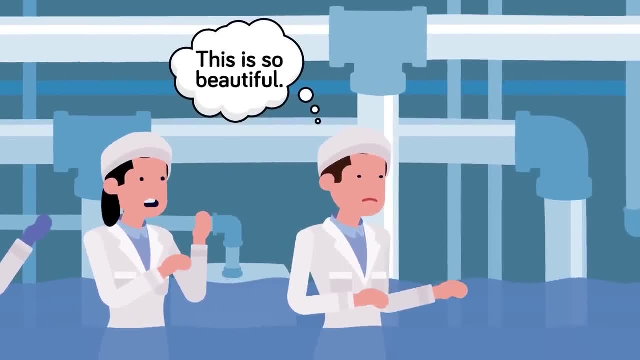 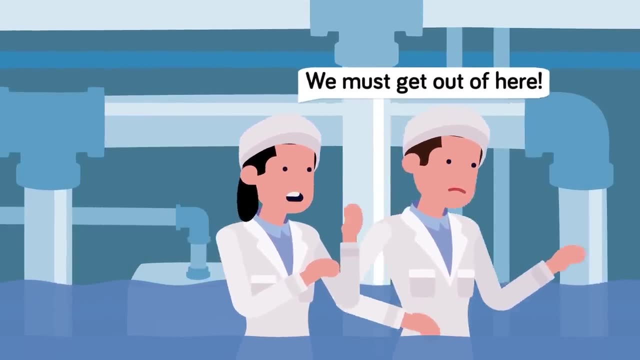 and he sees something magical: a great beam of light reaching to the heavens. It's magnificent and beautiful And, as things now stand, Alexander is not aware of how deadly it is. For a few seconds, he just stares at. what he doesn't know are gamma rays and neutrons. A more experienced colleague, 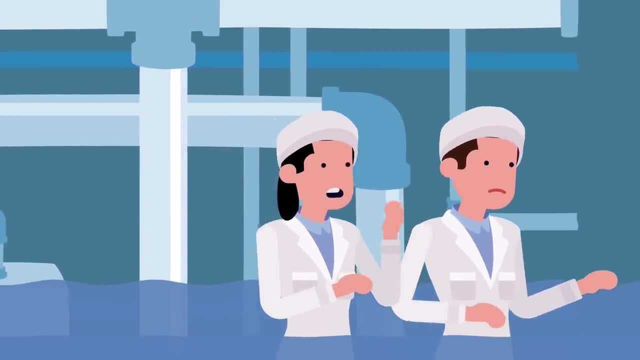 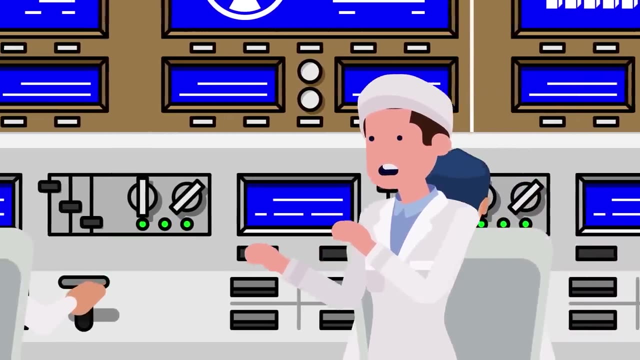 who knows what it is, grabs him by the shoulder and pulls him away, likely saving his life doing so, Alexander sets off to Control Room Number 4, and there he meets the other guys who have been ordered by Dyatlov to go to the reactor hall and lower the control rods by hand. 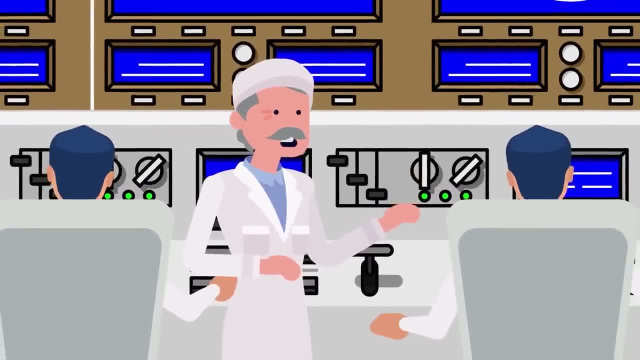 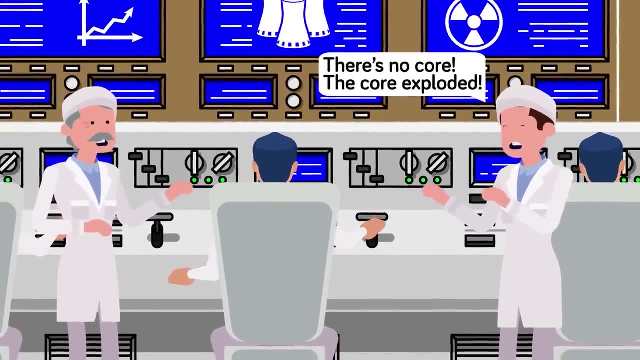 This is madness, sheer madness. Alexander screams. there is no reactor hall. The reactor has blown up. There are no control rods. They've blown up too. There's nothing left but space. The guys think he's crazy. Reactors don't explode. Alexander has to admit what he's seen. He's only seen from. 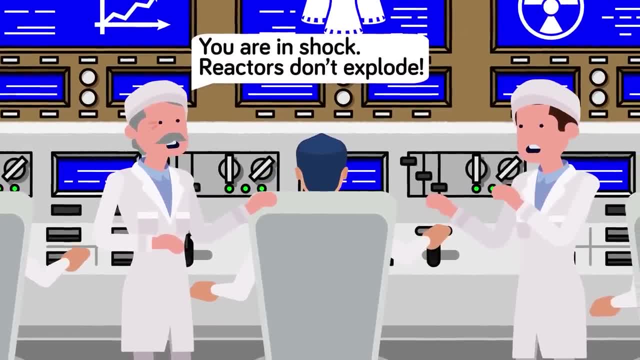 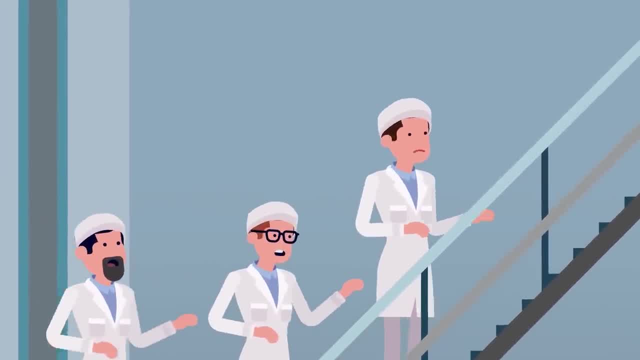 the bottom floor. The men tell him he needs to assess the damage from above to really know what's happened. The four of them head to the reactor hall, upper floor. Little do they know this is a journey to the end of the night for three of them anyway. As you know, Alexander only survives. 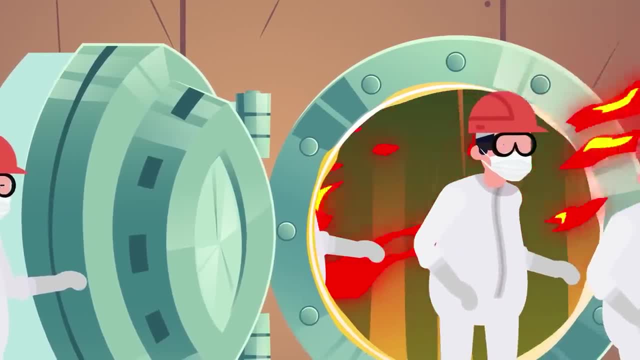 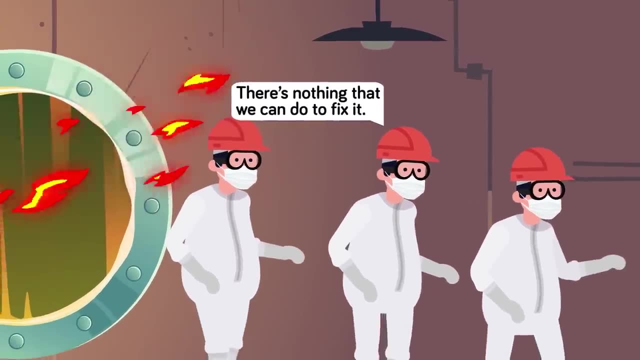 because he's the one that holds the door, being the strongest of the four. When the guys come out, they say nothing can be done. They look at Alexander and tell him he's right. They say the reactor hall now looks like a volcano crater. They understand that radiation levels are high. 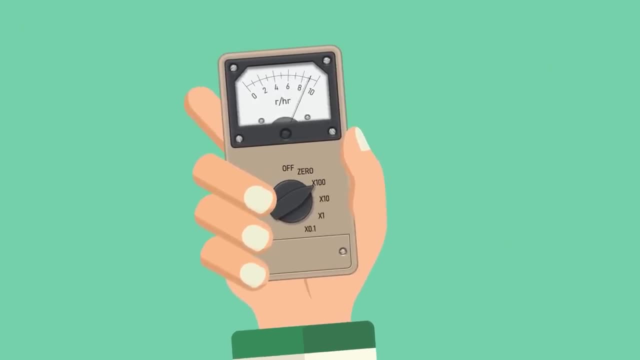 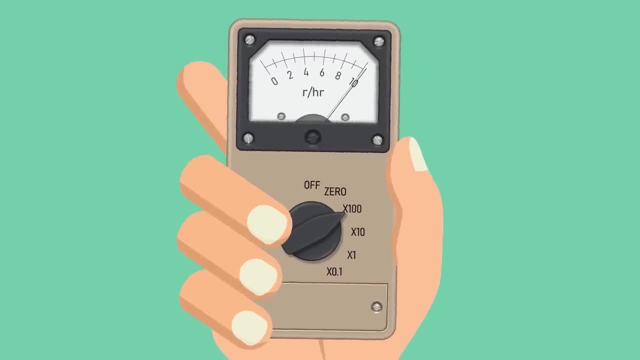 Of course they do, it's their job, But they don't know just how high. They look at the radiation level reader device. they have the dosimeter and that needle is off the scales, But they still don't know how bad they are, because what is happening is so unprecedented. It's still only 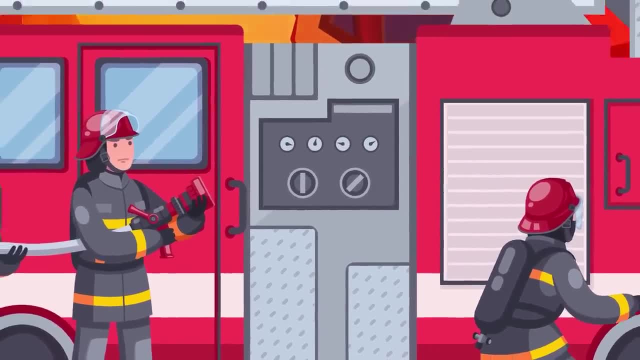 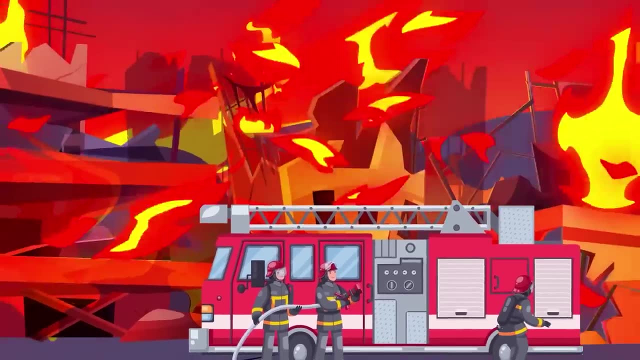 just after 1.55, but the firefighters are already outside on the scene. They too don't have much of an idea of the gravity of the situation. They don't know what's going on. They don't know what's going on And they start and try to put out some of the fires that have started in various 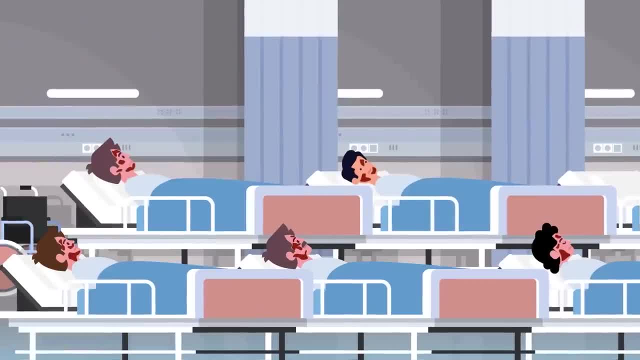 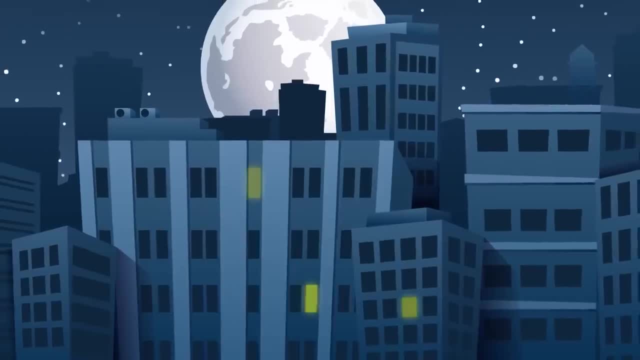 places. They're not even wearing protective clothing. Some of them will die in agony very soon. Others will pass away in a month, their immune systems destroyed by the radiation. Back in Pripyat, most people are in bed asleep, although a few are now standing outside. 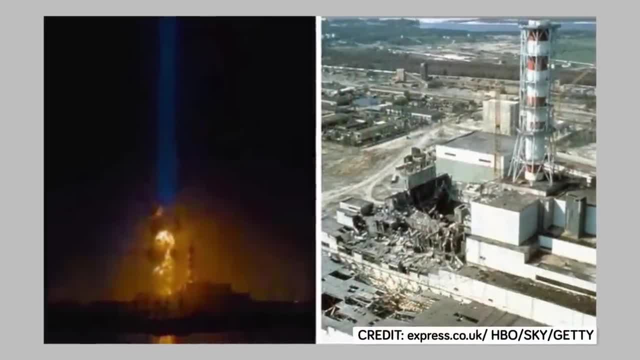 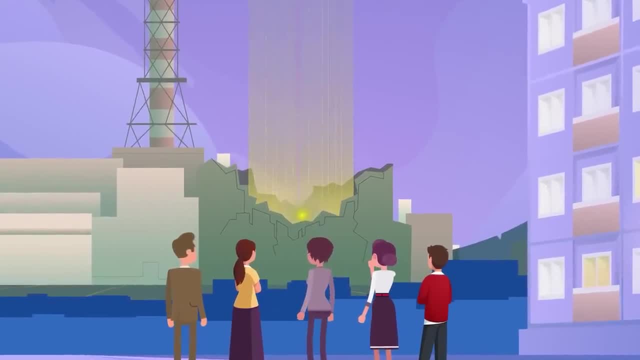 mesmerized by the ethereal beam in the sky they don't know is caused by irradiated air. They just think it looks cool. In the years to come, stories told in the west will say there was a large group of them on a bridge watching radioactivity. 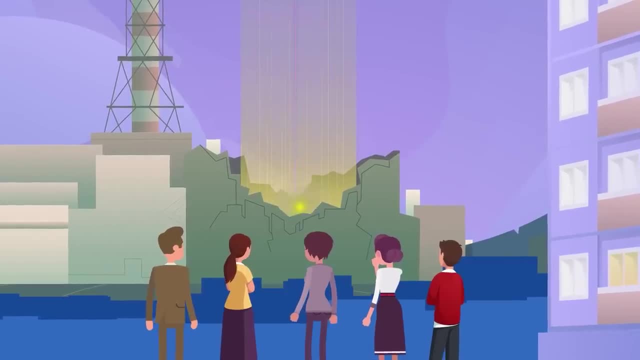 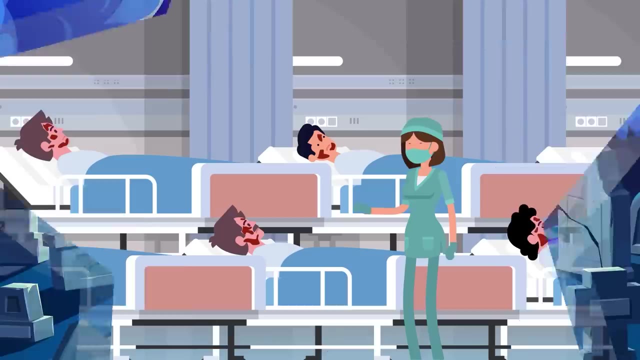 Blue dust fall like snowflakes. This will be called the bridge of death. The stories will say they all died, but none of that is true. There was no bridge of death. Most people were asleep at the time. In the end, most people who actually were close to the accident were 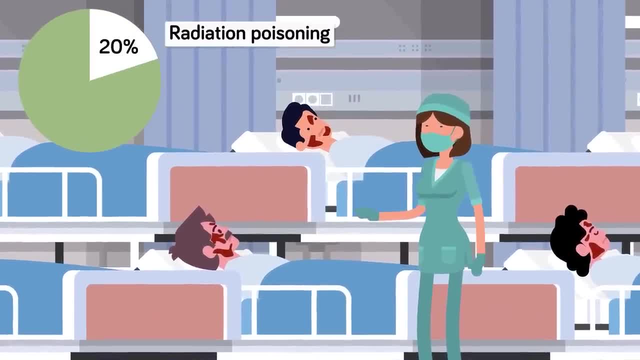 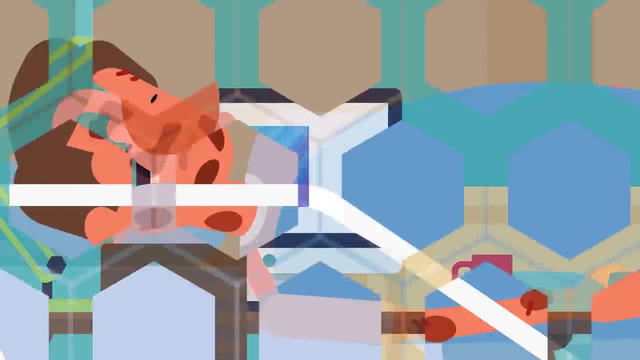 covered, with just 20% of those who suffered acute radiation poisoning biting the dust. As you'll see again in this show, it sometimes pays not to believe everything you see on TV or in the newspapers If you don't know the way radiation poisoning works on the body is 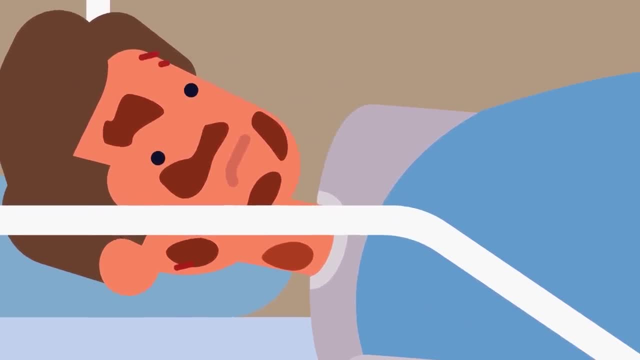 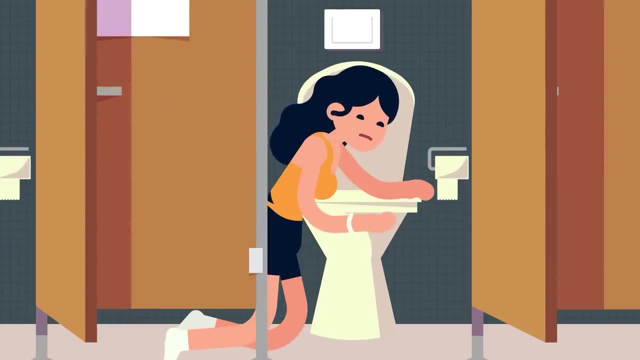 it takes out electrons from atoms in a person's molecules, destroying the chemical bonds and thus damaging tissue. We don't need to tell you that this is not good for the person. In short, after an hour or two, diarrhea and vomiting can occur as tissue in a GI tract breaks down and bacteria is let loose. 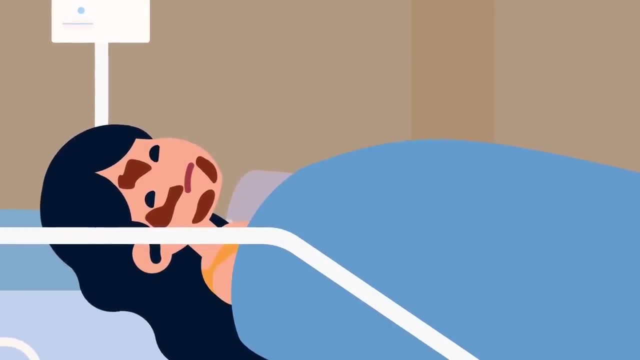 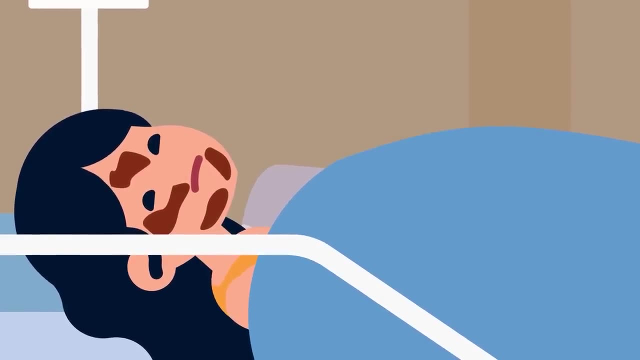 on the body, Bone marrow stops producing white blood cells and infections can't be fought, Since the person's immune system is incredibly weak. without an immune system, your countless bacteria eat you from within. This might take some time, so, even though the 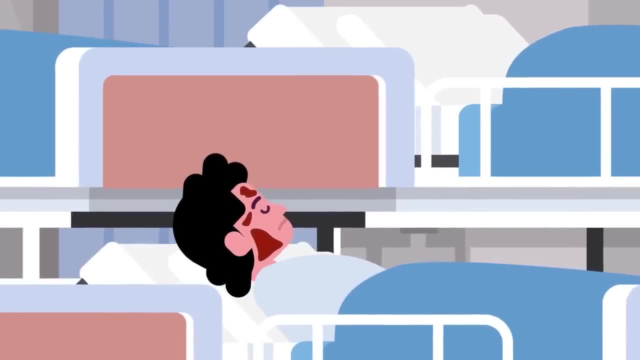 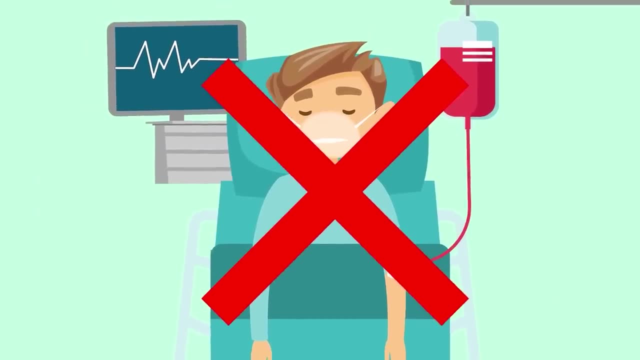 person is covered in blisters and ulcers. they could start to feel okay after a couple days, But then a blood infection might lead to a deadly sepsis. For some at Chernobyl, even a blood transfusion and bone marrow transplant won't help them. 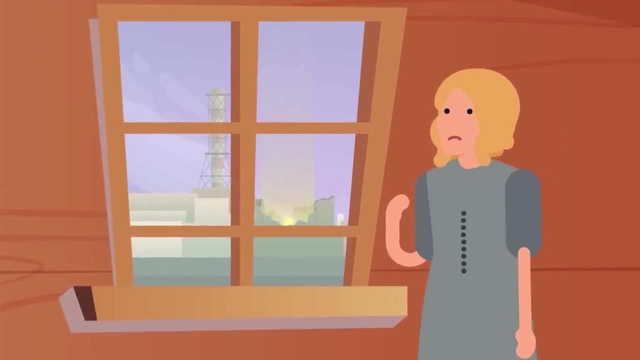 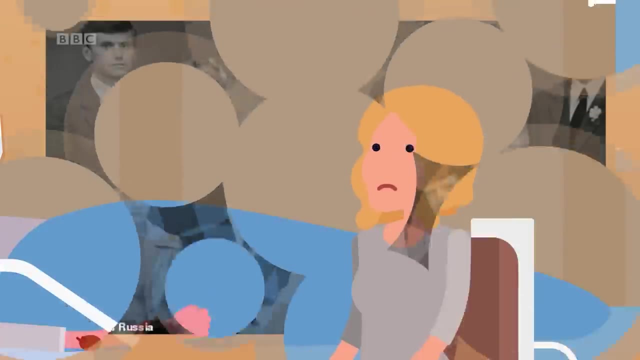 One of the townspeople is Lyudmila Ignatenko. She's already awake and has seen the glow. Her husband, Vasily, is currently fighting the fires. The two are due to have a child in two months. Fast forward a week and his skin is covered in boils, and when he turns on his pillow, 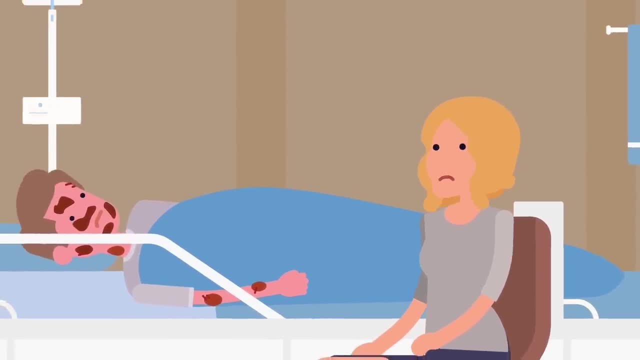 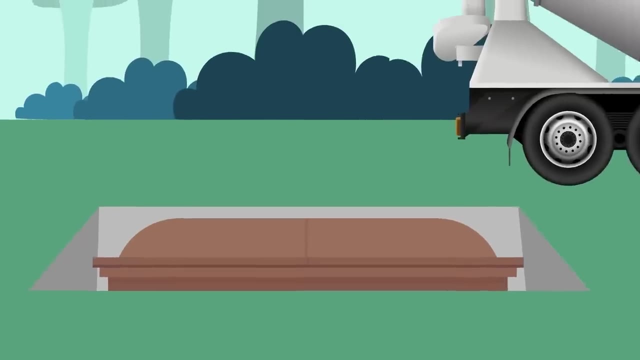 he leaves skin and hair behind The lesions spread out, and some of his skin now looks like a white film. At one point he asks Lyudmila for a mirror, but when he sees his own disfigured face he cries out in horror: Vasily will be buried in. 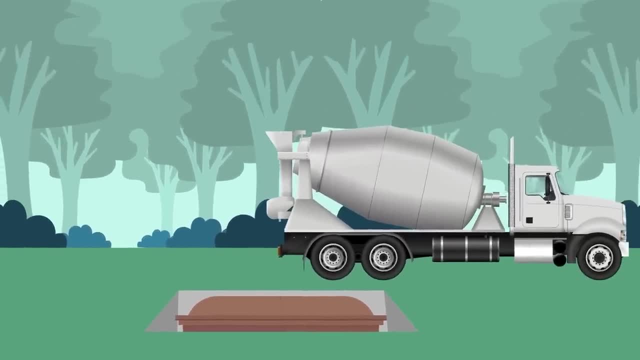 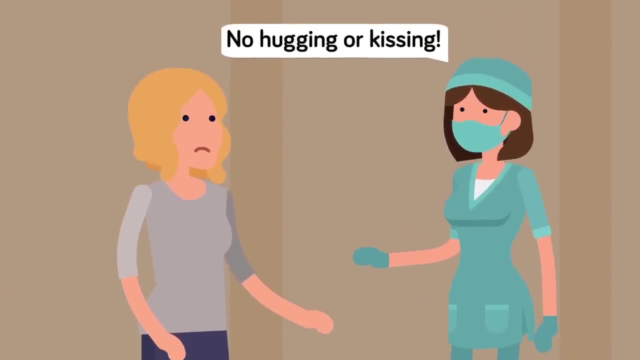 a zinc casket under cement, his body still radioactive. Lyudmila is lucky she even got to see him. A nurse told her it was too dangerous. She looked at Lyudmila and warned: if you start crying, I'll kick you out right away. No hugging or kissing, don't even get near him. 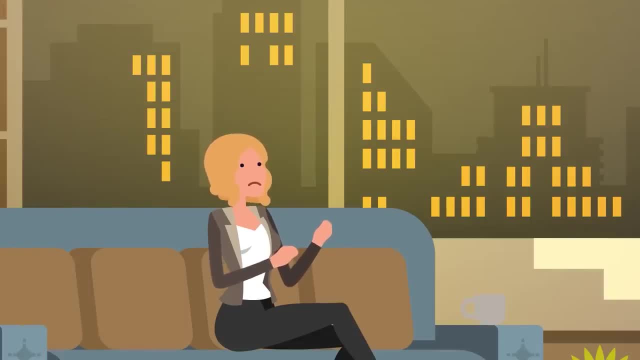 You have half an hour. Lyudmila will have much to say about this in time to come. She'll also lose the child. It will be born with a congenital heart defect and liver cirrhosis and will die after a few hours. 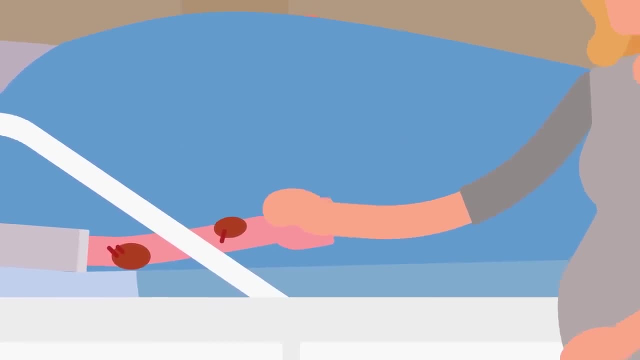 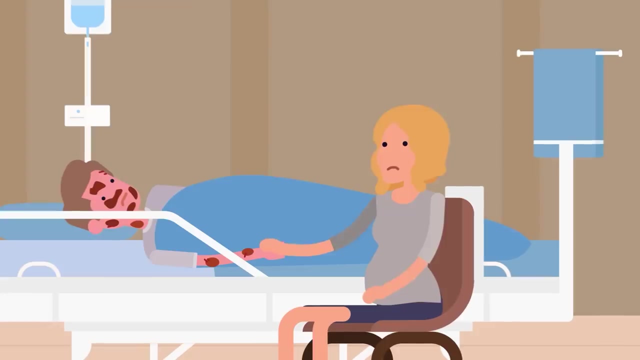 People will criticize her for this, asking why she visited her dying husband. The radiation from him contaminated her and the fetus. they'll say: But you can't just catch radiation from a cleaned person and there's no proof this is how the baby died. A falsity that 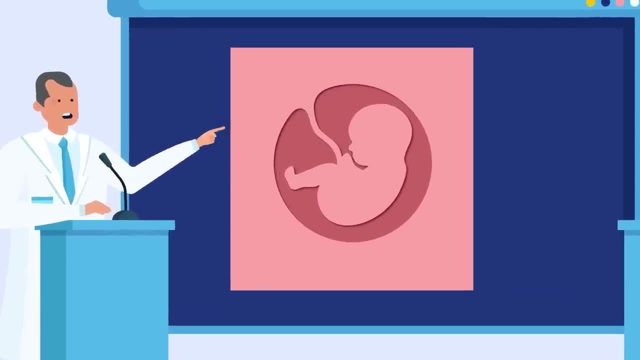 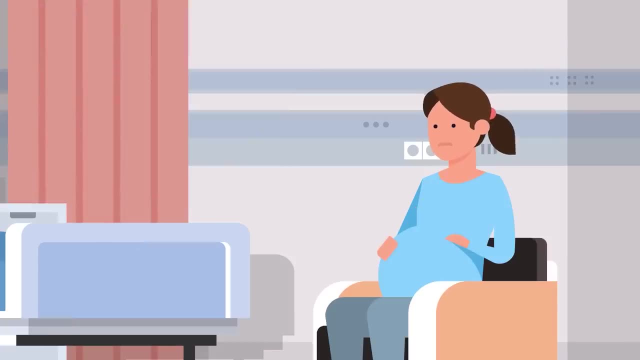 will be talked about for years is the baby somehow took the radiation and that saved her. This is not scientific at all, but it makes a good newspaper copy and great TV. The consequences of this misinformation will mean the lives and lights of hundreds of thousands of babies. 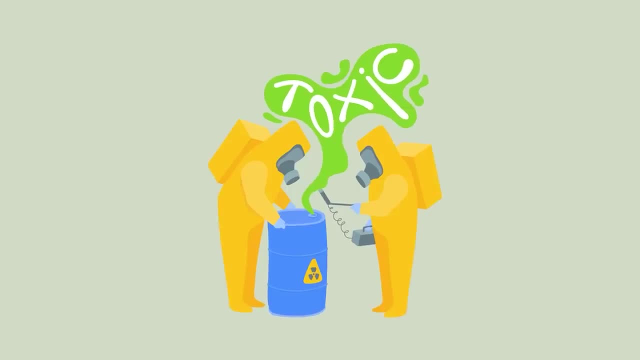 are put out before they get going. It's interesting, though, that, while seeing her dying husband wasn't the reason for the baby dying, it was very likely radiation exposure from somewhere else that led to the death. Back in 1986, the nurse that told Lyudmila not to touch her husband couldn't have known. 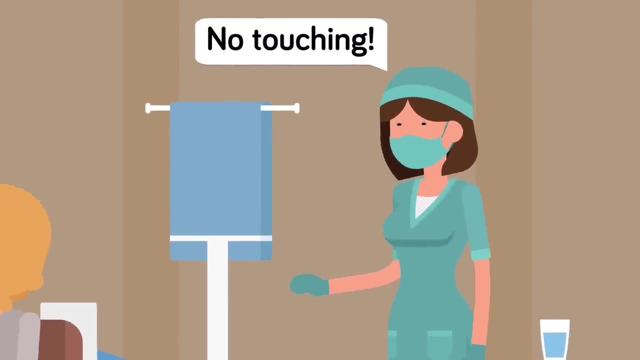 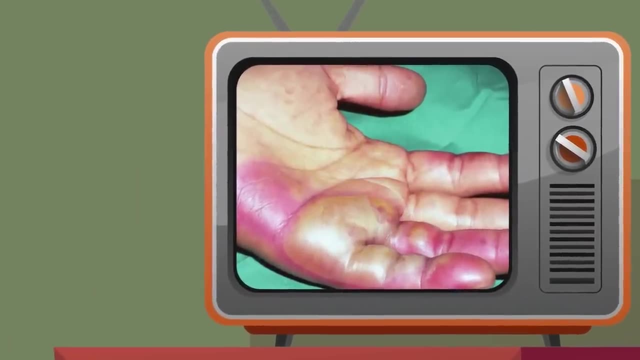 radiation doesn't spread to people after they've been cleaned and are out of their contaminated clothes. It's not contagious. We should also tell you that a person's hand can't suddenly burn when they touch the hand of a contaminated person. That's TV, not reality. 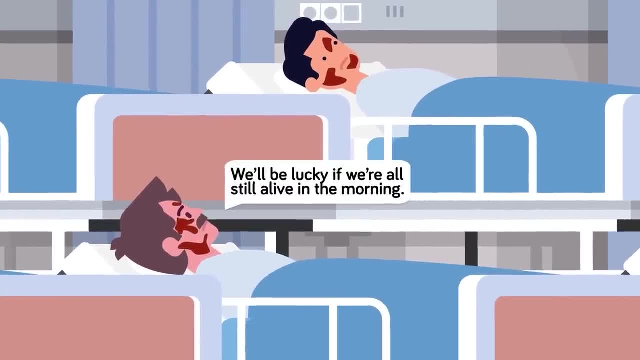 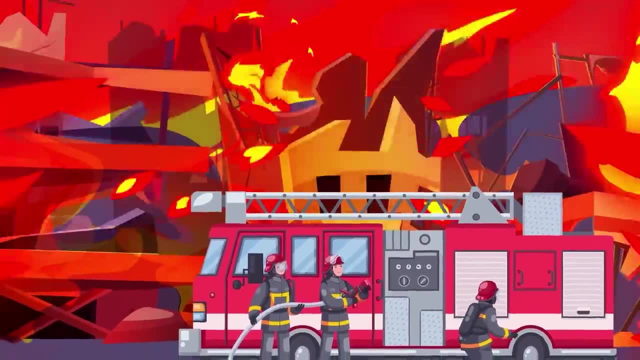 One of the firefighters turns to his friend and jokes saying: There must be an incredible amount of radiation here. We'll be lucky if we are all still alive in the morning. As the survivors will later testify, they were never told the reactor was on fire, only that there were regular fires to put out. Some of them kicked the. 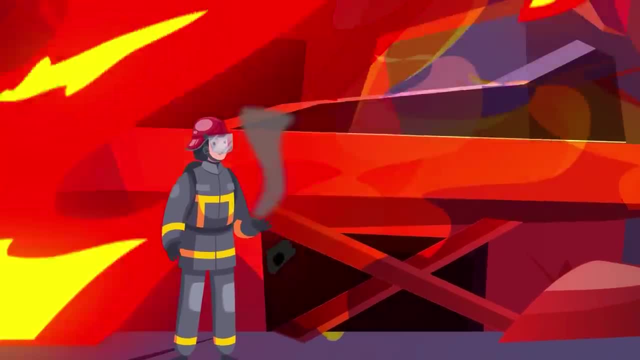 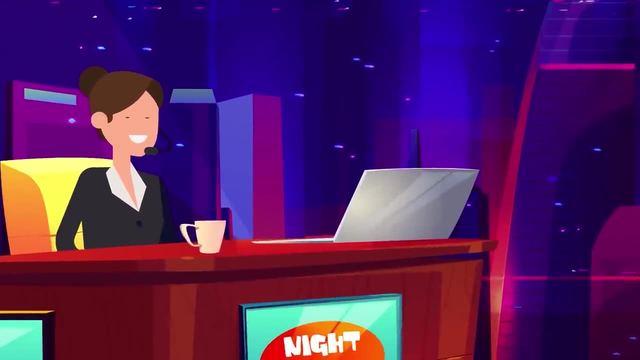 radioactive blocks, even picking them up with their hands after they'd doused them. They would have never done those things had they known the truth. One of the firefighters who survived explained how little they knew, saying some of his colleagues went up to the roof to work from there. Soberingly he said, then those boys who died went up. 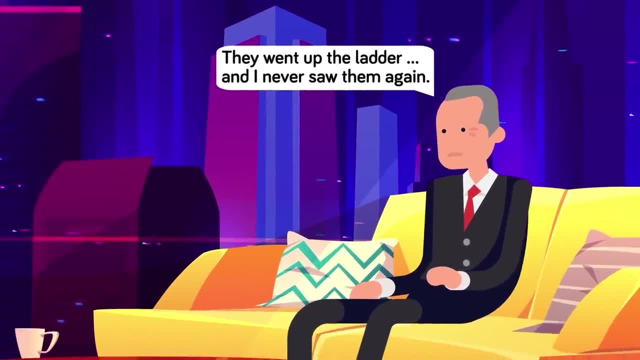 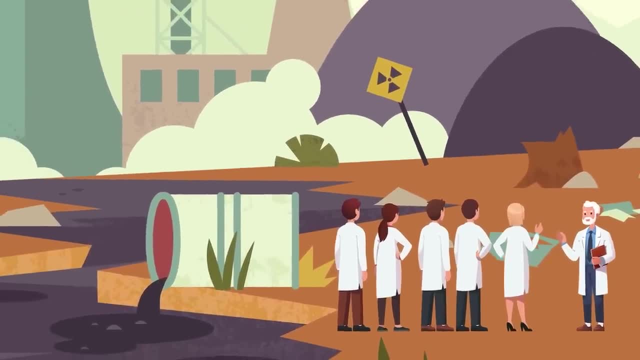 to the roof. Ashchik Kolya and others, Volodya Pravik. they went up to the ladder and I never saw them again. Hour 3: Local officials have already arrived on the scene to discuss what's happening When they're. 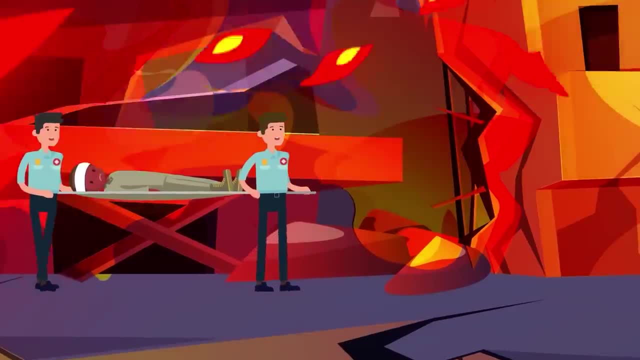 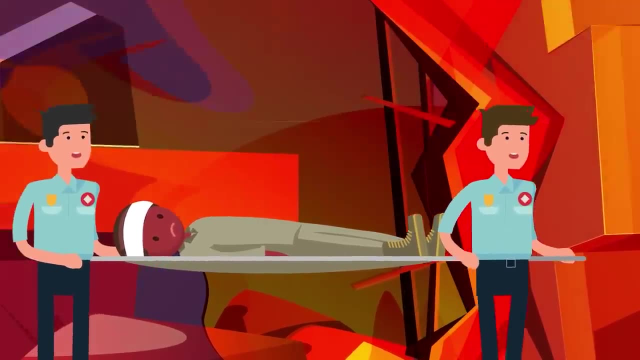 told. they're not told the entire truth. That's because only a handful of people right now truly understand that the reactor has blown up and some of them are now burned, vomiting, So not in a meeting explaining what they've seen. Dyalov still thinks what he always has: that a water tank has blown up and the radiation. 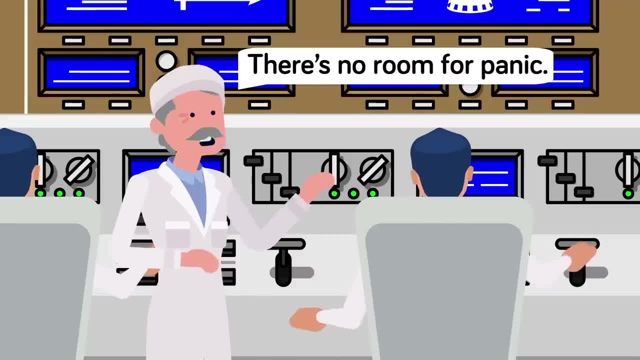 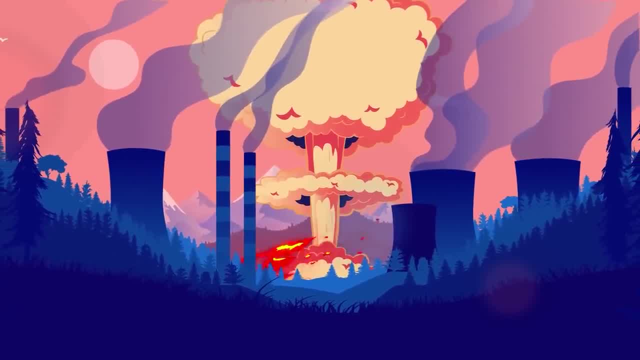 currently making some people very sick is from contaminated water. He just can't believe that the core would blow, even though some people are starting to realize that a water tank blowing up wouldn't lead to so much destruction. Hour 4: More firemen arrive to help with the fires. The last thing anyone wants is Reactor 3 to 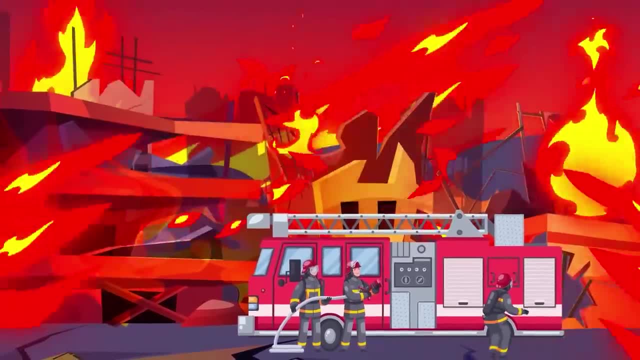 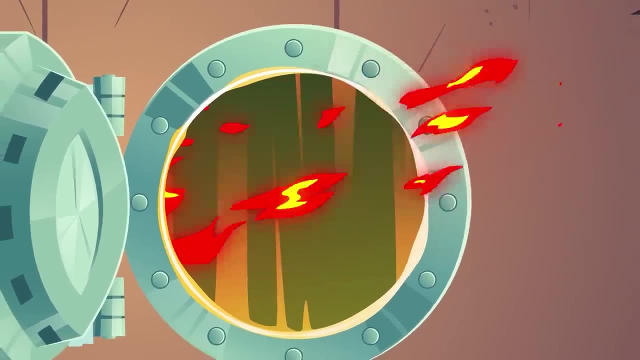 set on fire, which is looking like a possibility. It's soon safely shut down, but Reactors 1 and 2 keep going until the next day. Inside Reactor 4 is now a molten reactor core, a large graphite and concrete slag that's burning at around 1200 degrees Celsius. 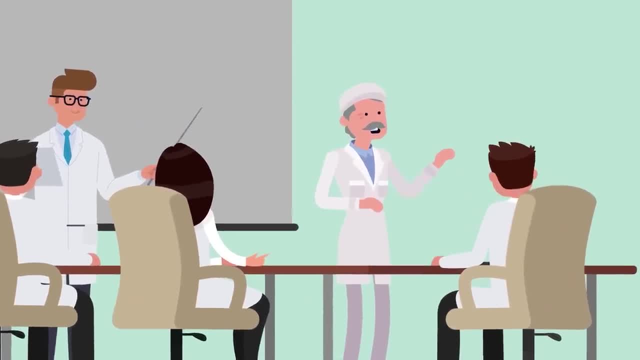 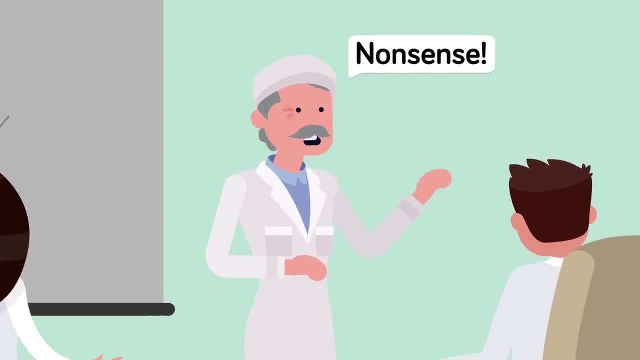 Hour 5.. Another meeting is held now with experts. Some ask about the high levels of radiation, proffering a theory that the core might have blown. Nonsense, says Dyalov, even though he's not far from keeling over himself A second later. 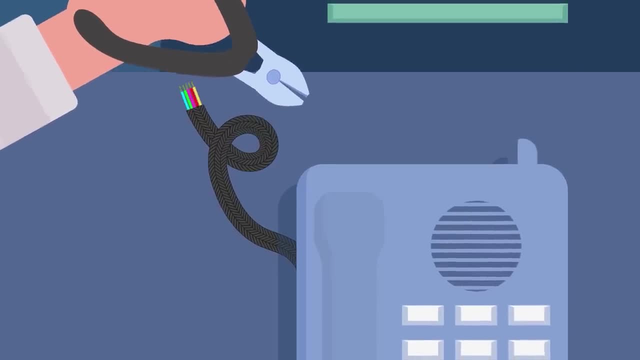 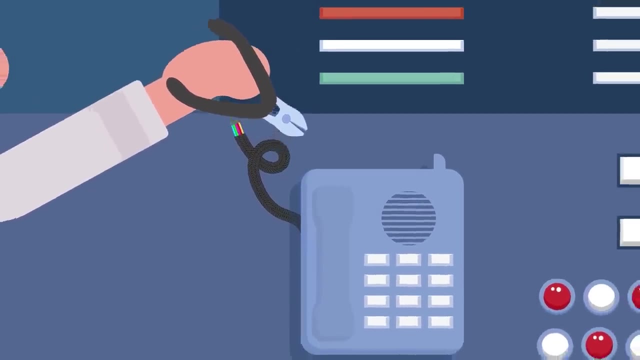 he throws up, A decision is made that no one will leave the town, Not yet. Perhaps they can be evacuated in three days. All the phone lines are blocked in case anyone starts spreading rumors- which one official calls misinformation- that can negatively affect the Soviet Union Police. 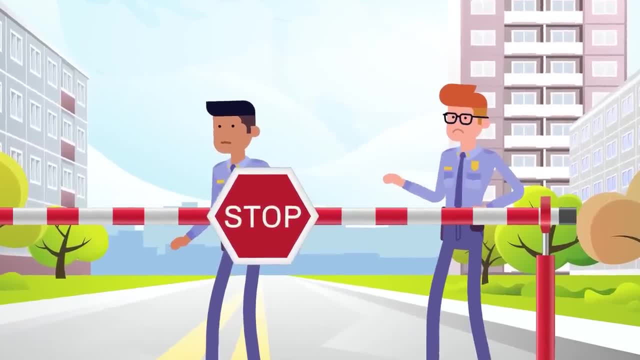 soon start blocking roads, just as soldiers pass them on their way to help Hour 6.. The first thing Dyatlov says is that he's not sure what's going to happen. He's ready to start a fire. He's ready to help with the cleanup job. 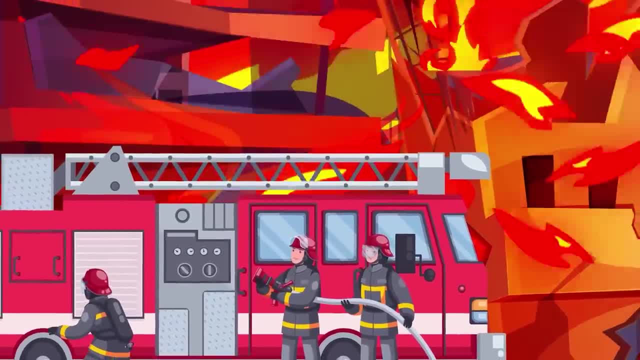 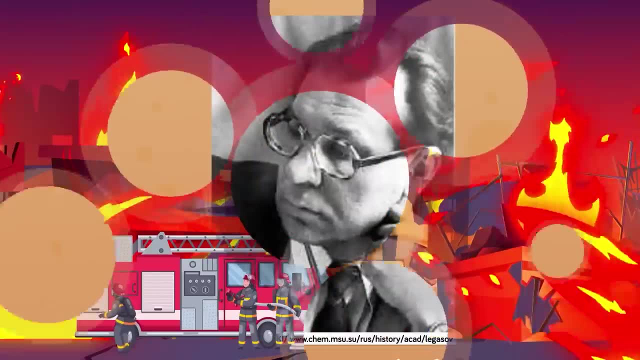 Hour 7.. At 6.35 am most of the fires are out, But by no means does this mean the problems are over. They're only just beginning. Real horror is taking place inside that reactor. A man who understands this horror is Valery Legasov, the deputy director of the Kurchatov Institute. 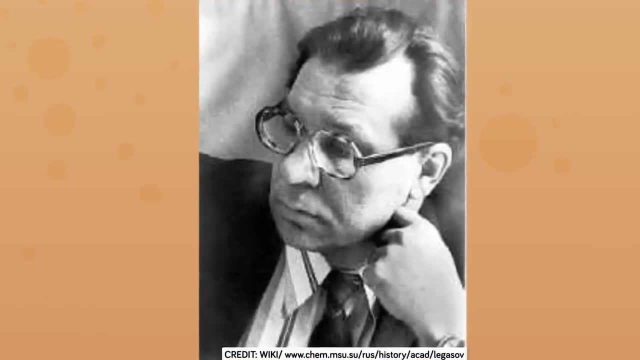 of Atomic Energy and the man that will lead the commission to deal with the accident. He will also be the one that testifies during the tribunal and, as you'll see, he's the guy that exposes the Soviet Union's shortcomings when it comes to producing nuclear energy. 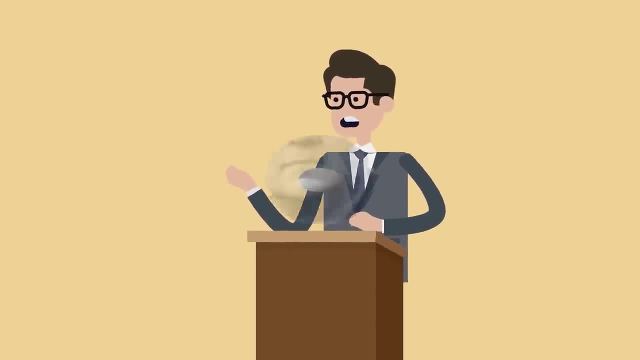 He's also the one that'll be the one to testify during the tribunal. He's the guy that exposes the Soviet Union's shortcomings when it comes to producing nuclear energy. Hour 8.. He's called on the phone Soon. he's at the airport with the man who will manage the. 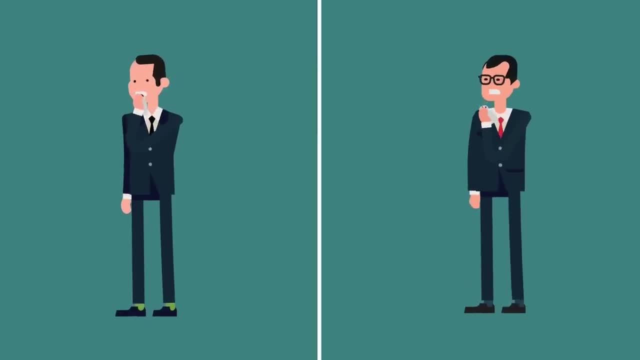 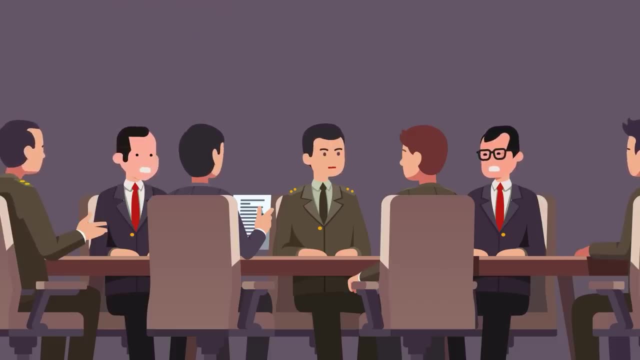 crisis, Boris Cherbina. In time, both these men will suffer from radiation poisoning, but for now they still don't know exactly what happened. Hour 13. It's around midday when they attend the meeting to discuss matters Legasov already knows. 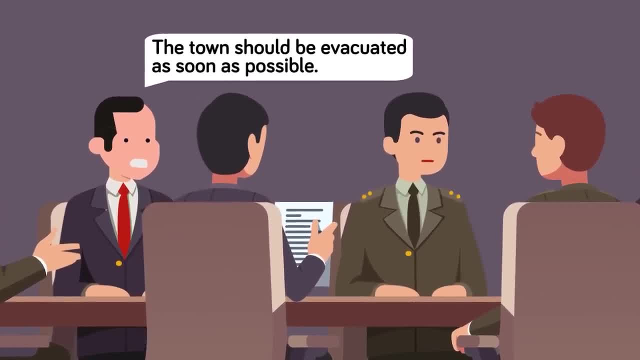 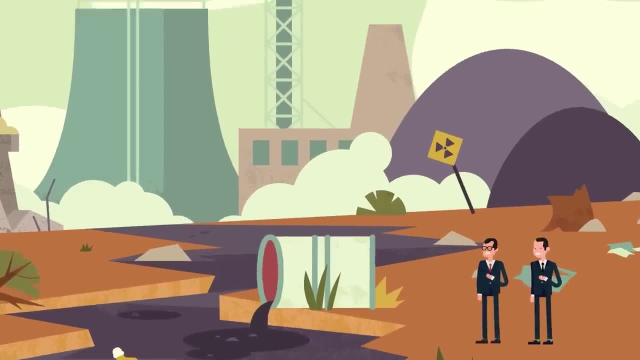 about the people in the hospital suffering from severe radiation burns. so he and others agree the town needs to be evacuated. Hour 30. Legasov is driven in an armored personnel carrier to assess the damage for himself. It's bad, very bad, He says they have. 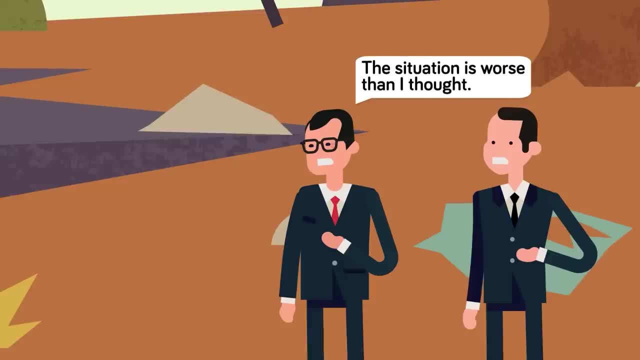 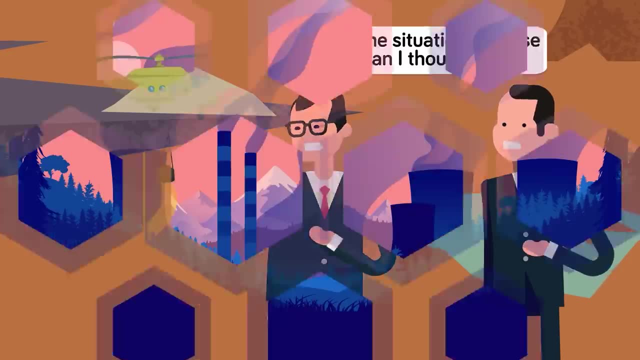 to get that main fire under control or radiation will be taken by the wind for many, many miles. Many parts of Europe, not just Ukraine, are at risk. This is a disaster of unbelievable proportions. It's agreed that dropping sand and boron on the reactor. fire from helicopters might be the best. 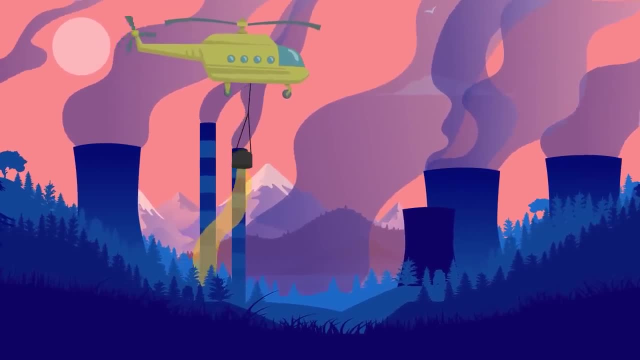 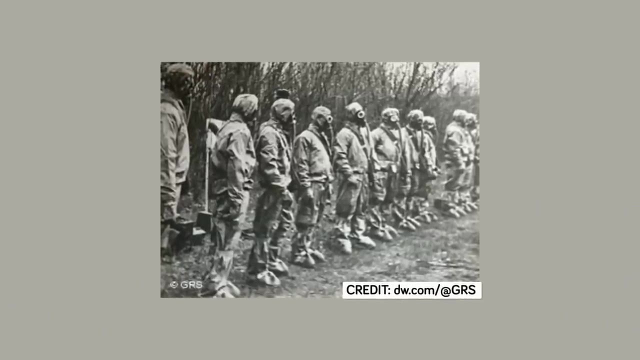 way to go, even though Legasov knows it might not work. They have no choice. he says Something needs to be done right now. The military will help with the cleanup and many men will be expected to risk their lives. These people will become known as the liquidators, and many of them will suffer long-term health. 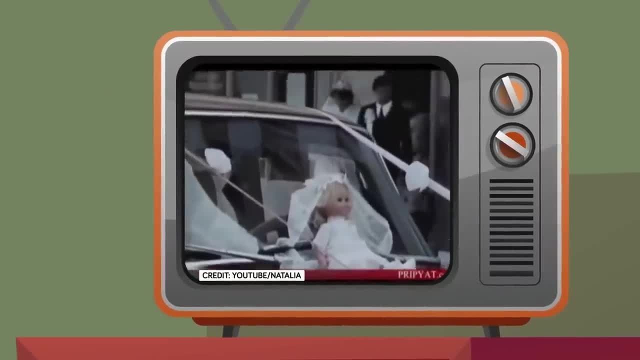 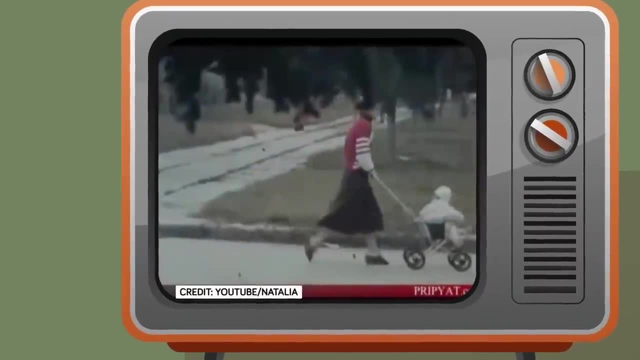 effects from their work Hour 33.. Sharabina gets on the phone with Moscow and reports: we've measured the radiation. Pripyat needs to be evacuated immediately. The station is close by and it's emitting radioactive contagion, and people in the city are living it up full blast. 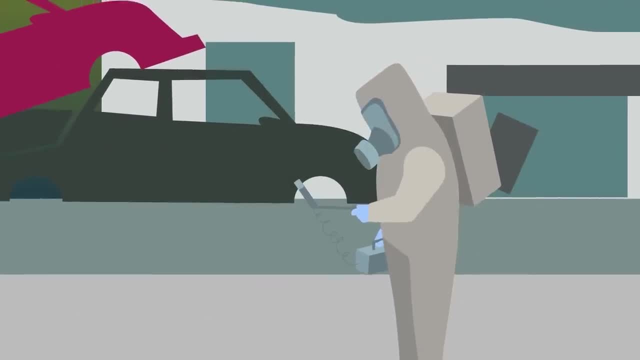 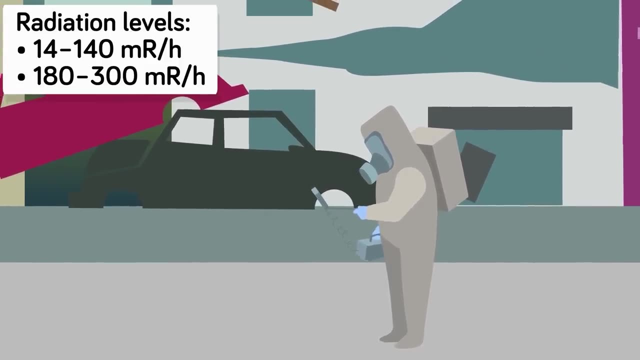 Weddings are going on. Levels of radioactivity in the town are rising at an alarming rate. Earlier in the day the level was between 14 and 140 milliroentgens per hour, but that's gone up to 180 to 300 milliroentgens and in areas closer to the plant, 600.. 50. 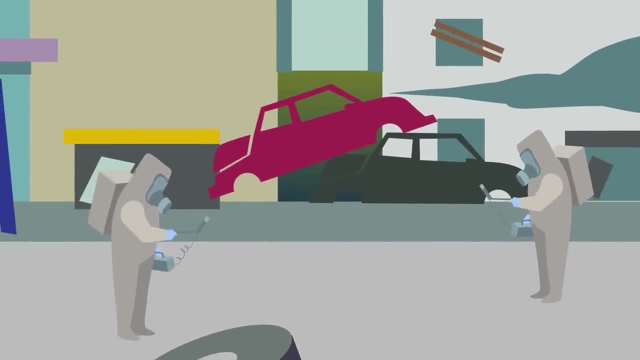 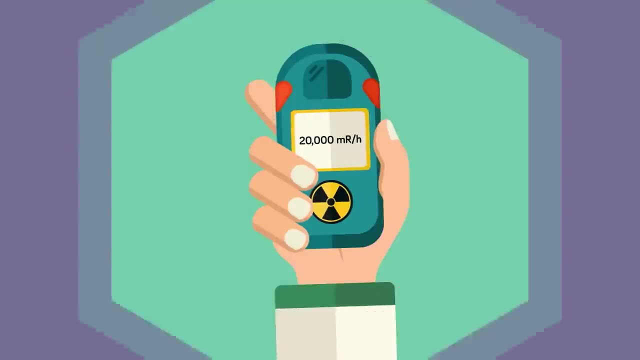 milliroentgens or more per year can be dangerous. with 400 milliroentgens per year killing you, The people in that town now have a much higher risk of developing cancer and they have no idea about it. Still, in parts of the plant, the level has reached an astounding 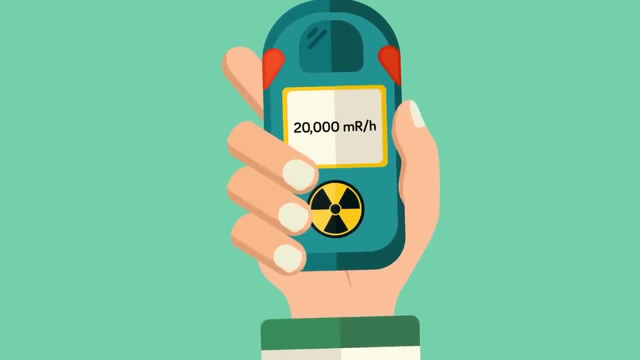 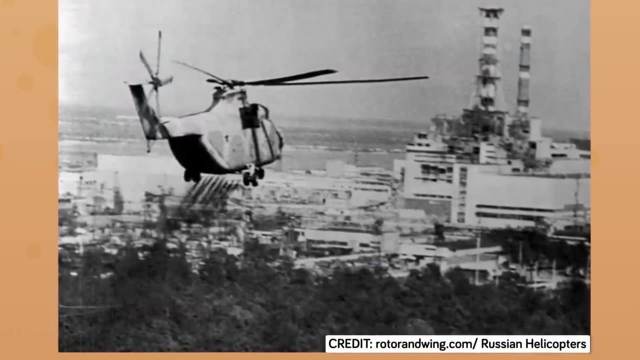 20,000 milliroentgens per hour, and that's why some men died so soon after exposure Hour 36.. Sometime in the morning the first helicopters start dropping the sand and boron on the fire. It's a perilous job. Getting too close to the hole where the reactor was can lead. 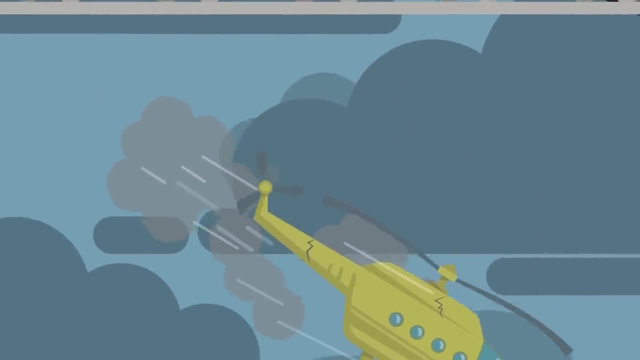 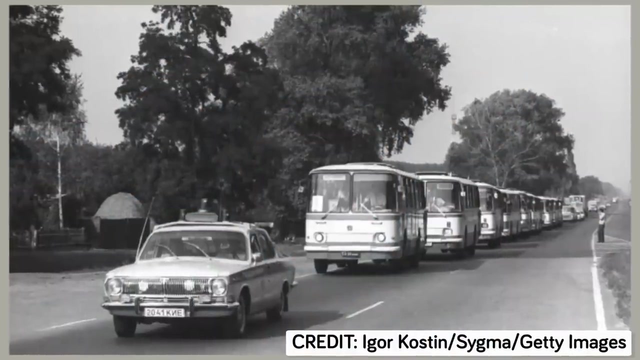 to acute radiation sickness. It's dangerous enough anyway, as can be seen when one helicopter collides with a chain and crashes, killing the men on board. Hour 38. The evacuation begins From speakers. all over the town comes a woman's voice. 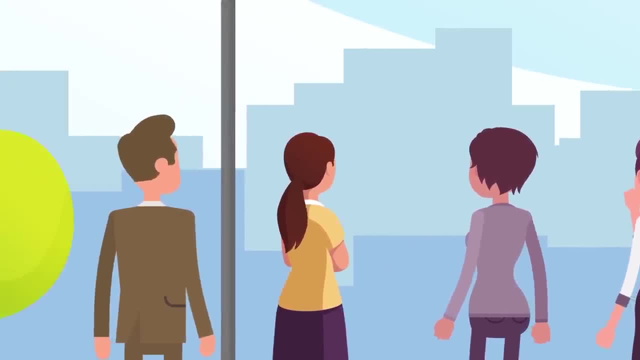 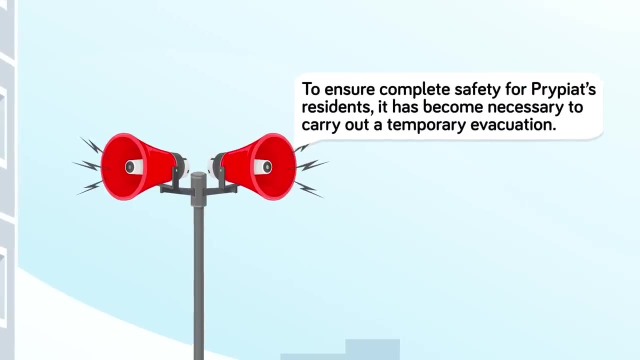 saying the same thing over and over again: Attention, attention. In connection with the accident at the Chernobyl Atomic Power Station, unfavorable radiation conditions are developing in the city of Pripyat. In order to ensure complete safety for residents, children first and foremost. 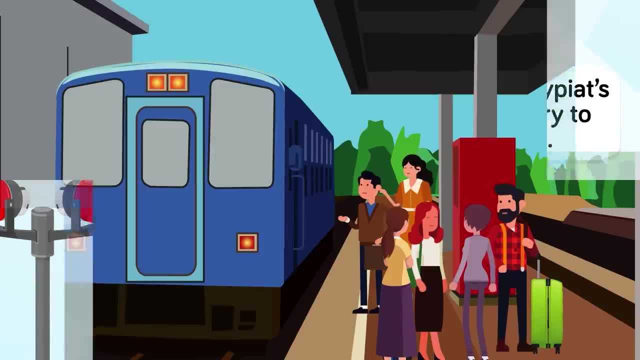 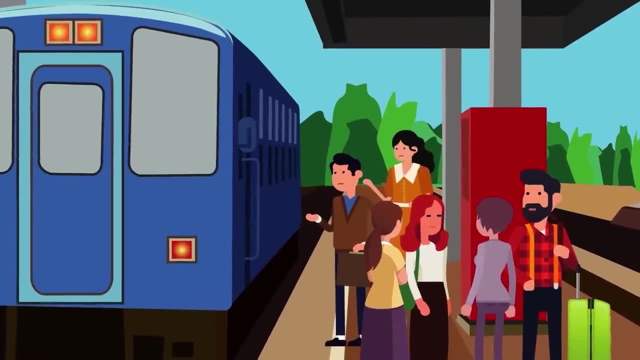 it has become necessary to carry out a temporary evacuation. They're told to take everything with them- that's important, including all their personal documents. They don't know it, but they're never going back to their homes. Just one hour before this announcement, 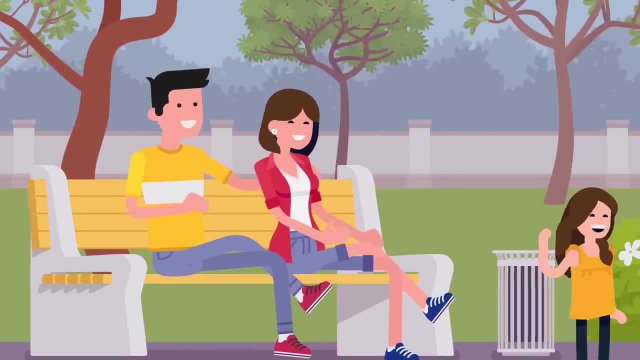 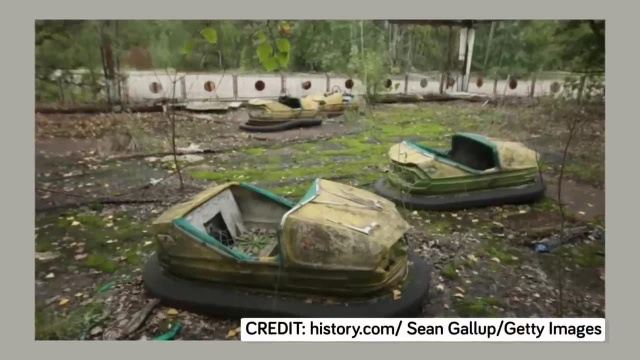 families were enjoying the weekend In the cafeteria in the shopping mall. kids and their mothers were hanging out and eating ice cream. For them it was just a normal day. There were kids playing on the bumper cars. Then suddenly they were told the ride was over. 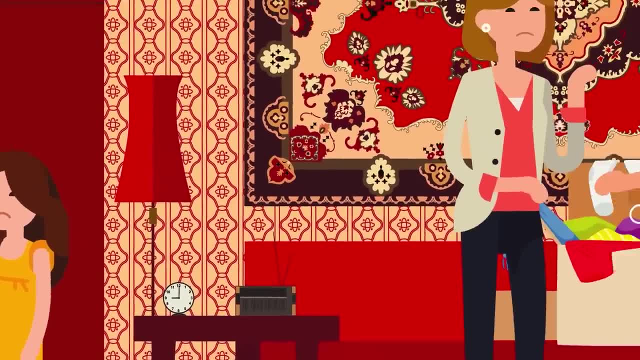 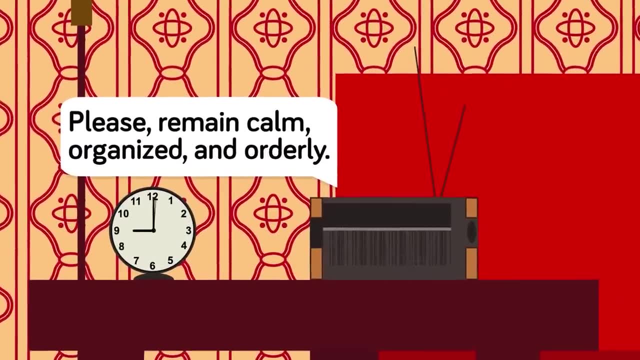 Now they're taken aback when they hear the speakers say: Comrades, on leaving your dwellings, please do not forget to close windows, switch off electrical and gas appliances and turn off water taps. Please remain calm, organized and orderly. What's startling is these people have not been told the full story. 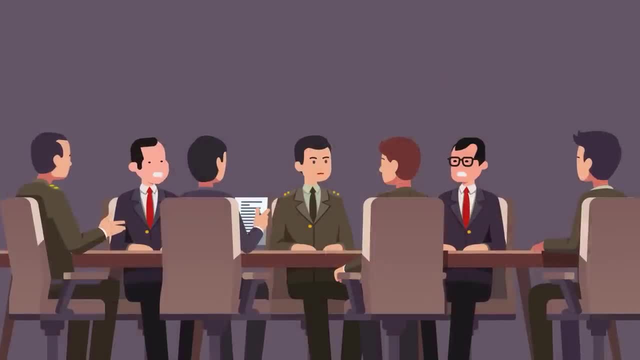 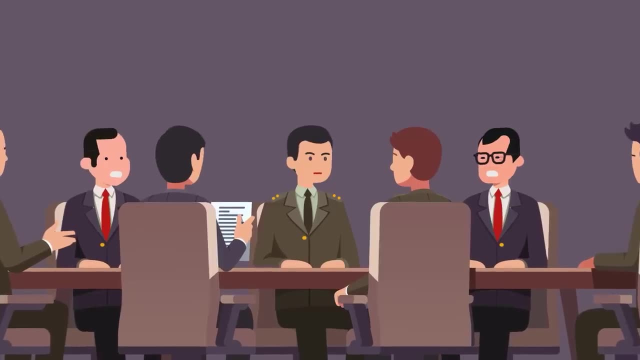 and certainly aren't given any protective clothing. In spite of the fact that Soviet officials know about the dangerous levels of radiation so far, they don't want to cause too much panic or for the word to get out about the disaster. Hour 42. Shcherbina calls Premier Nikolai Raishkov and explains: 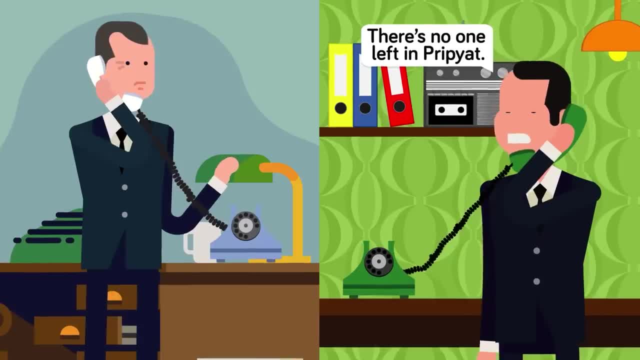 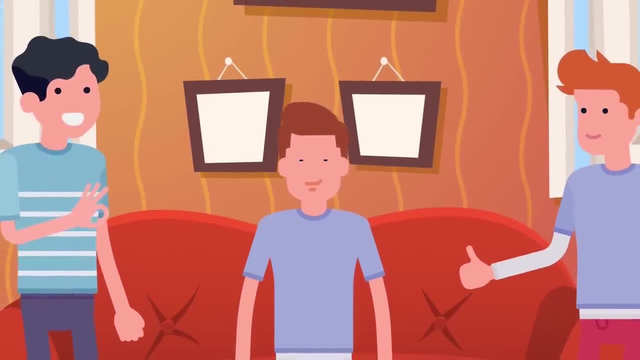 There are no people left in Pripyat. There are only dogs running around. What happens to the mutts in the end is awful, but that's a few days away yet. Shcherbina is not exactly correct about all the people leaving. Some young folks have hidden, so 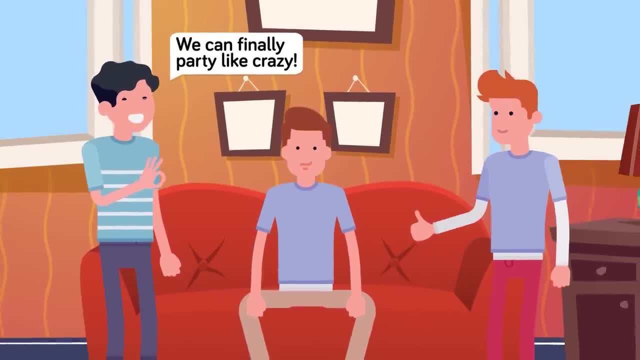 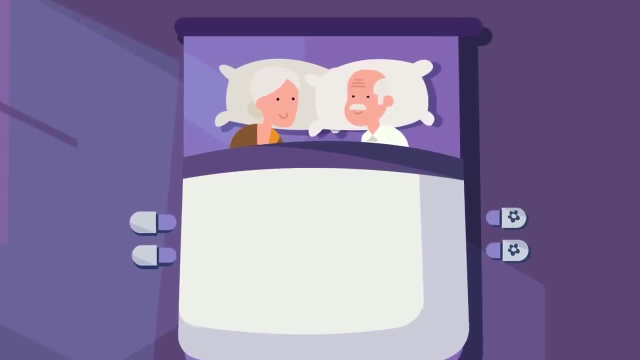 they can stay together in their parents' apartments and get it on for once with some privacy. They don't care much about some little radiation leak. Old folks too have stayed behind, or some of them have. They're well past the age of moving away and they're too tough to worry. about radiation. Some have lived well through wars, famine and Stalin's reign of terror. Hour 46. 116,000 people have left. About 1,200 have stayed behind, mostly the aged and many of them women, Babushkas as they say in Russian. 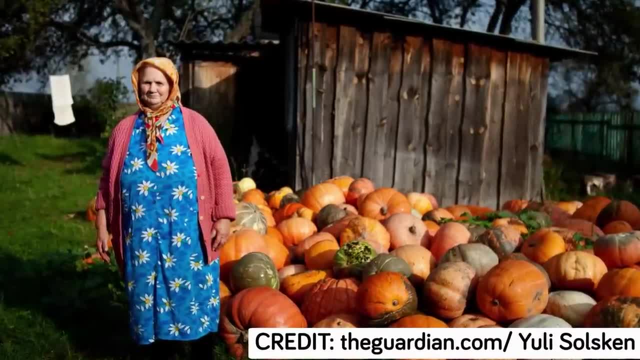 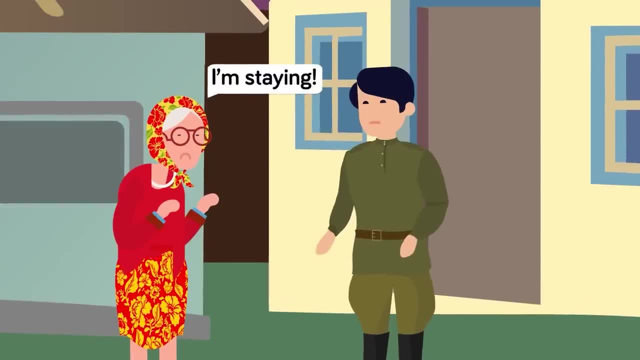 They have refused to budge. but it's hard to argue with a stubborn babushka. One woman, Hanna Zavarotnya, is given a stern order to leave after she's been found by a soldier. She looks him square in the face and says: Shoot us and dig the grave, otherwise we're staying. 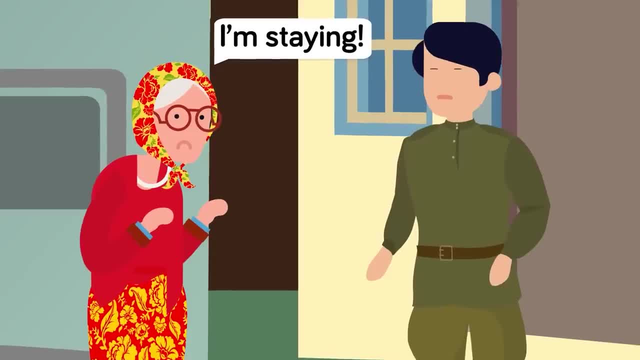 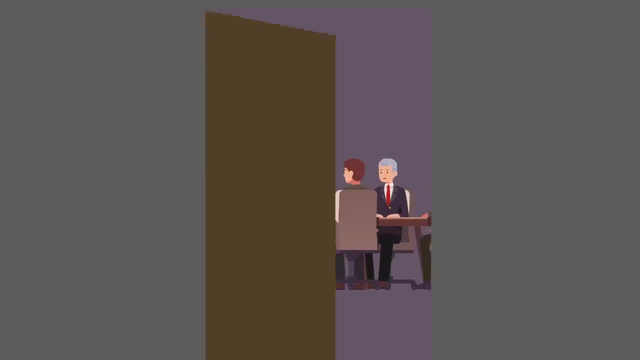 After listening to the soldier explain the danger, she replies: Radiation doesn't scare me, Starvation does. The world still doesn't know The extent of what's happened, and you can be sure the Soviet leaders are determined to try to keep matters within a fairly small circle. The KGB is told to stop the spread of panicky. 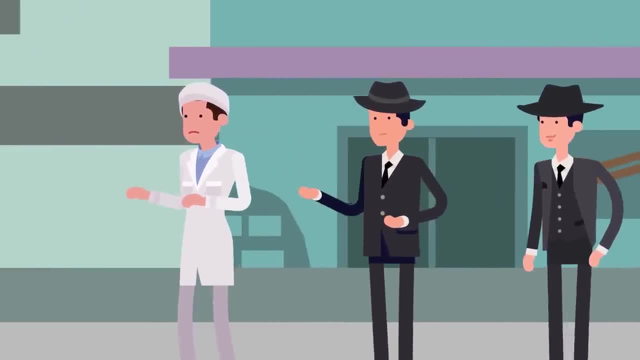 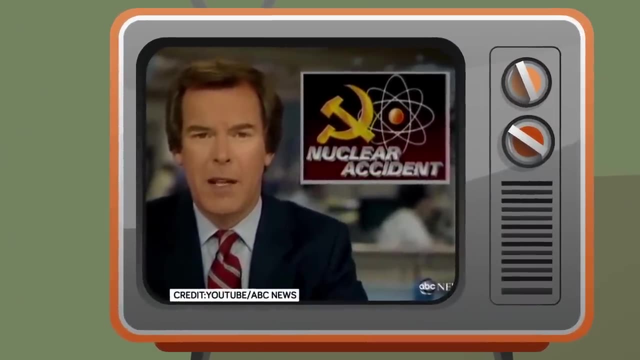 rumors and unreliable information getting out, although nothing they can do to prevent what happens. next Hour 52. The Soviets get word that Sweden has detected radiation and it has been identified as coming from Chernobyl. On top of this, soon the USA will have satellite photos. 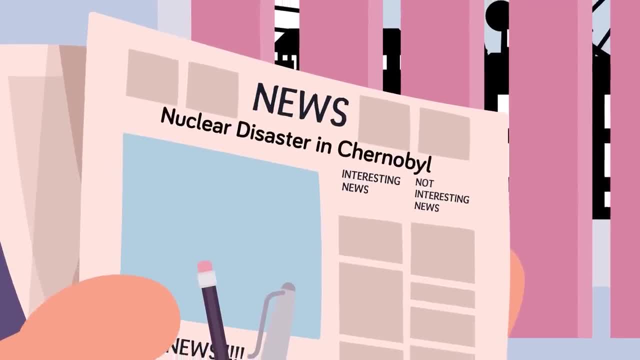 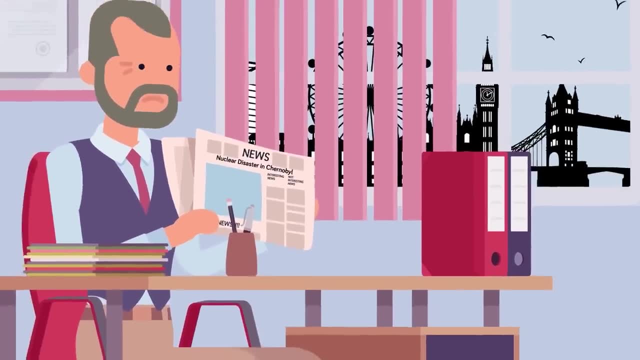 of the disaster. The news carries as fast as the radiation, with presenters all over the world telling people that this may be the case. The KGB is told to stop the spread of panicky rumors. something that's never happened before on this scale could mean dangerous radiation being 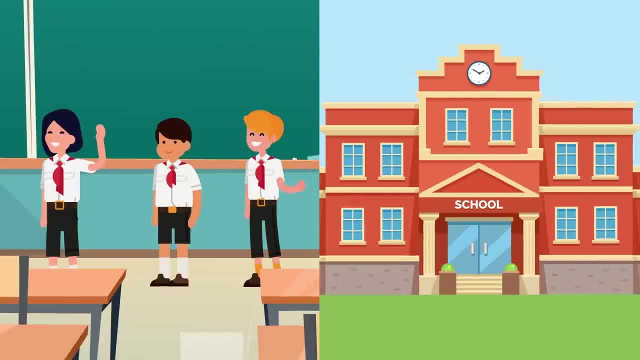 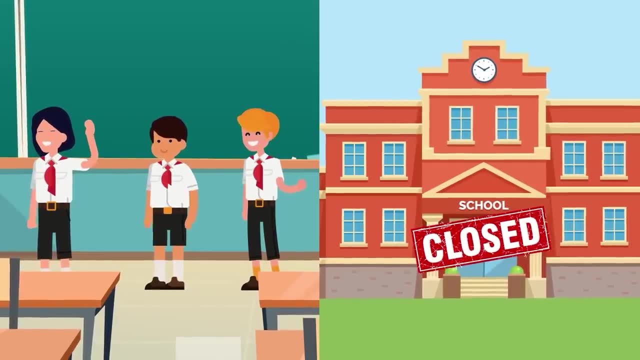 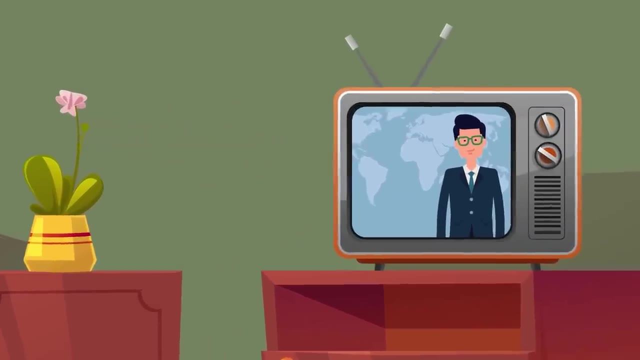 carried from Ukraine to other European cities. As the children of Chernobyl settle into their new surroundings, school kids in Germany are kept home in fear of radiation poisoning. Panic reverberates from North America back to Europe and into Asia. Hour 55. It's not until the evening that the official news is shown on Russian TV. 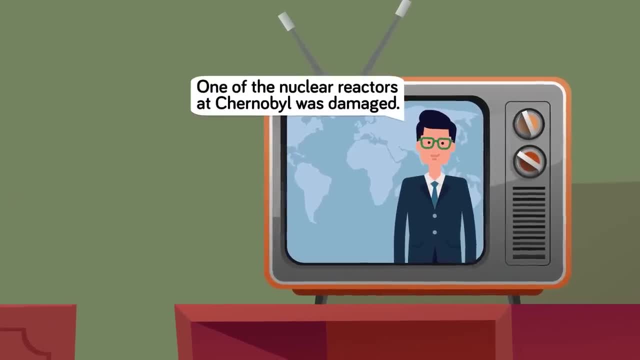 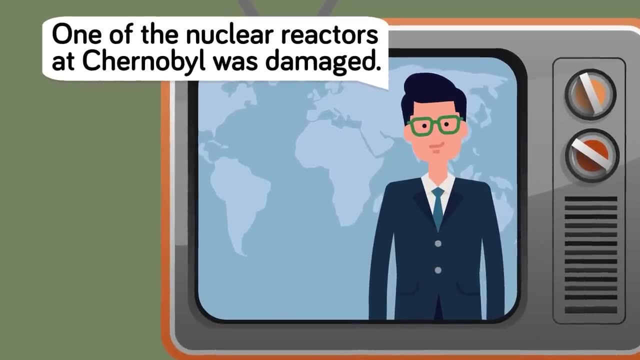 A report states there has been an accident at the Chernobyl nuclear power plant. One of the nuclear reactors was damaged. The effects of the accident are being remedied. Assistance has been provided for any affected people. An investigative commission has been set up. More Russian news follows, and this time with in-depth discussions, Not 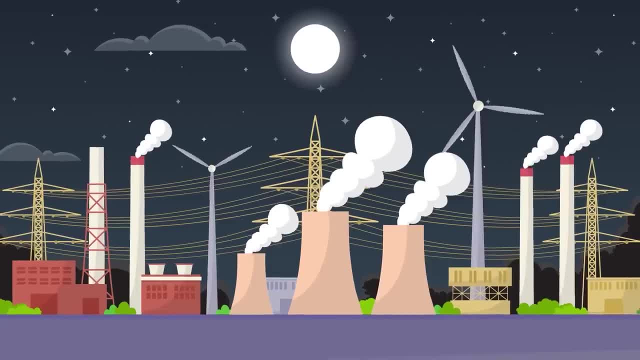 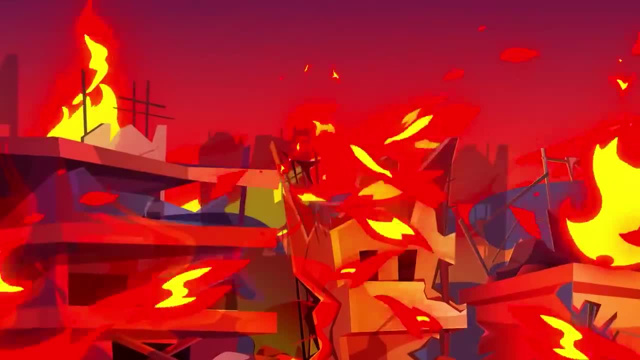 surprisingly, experts talk about the Three Mile Island nuclear accident of the USA and some other American nuclear mishaps. What the news doesn't talk about is what could happen at Chernobyl right now. A new kind of disaster could be in the works Hour 58. It was thought the water tanks were. 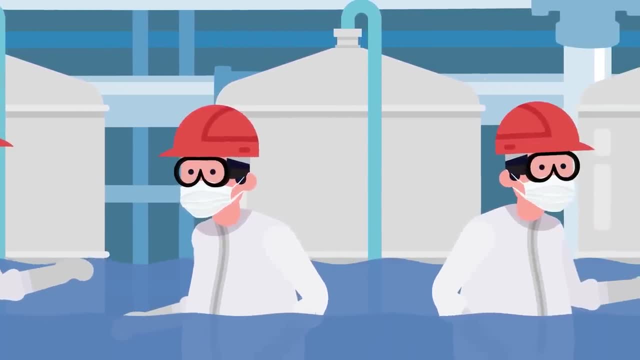 empty, which isn't actually the case. To make things worse, fire hoses have been filling the place with more water. Hour 58.. The KGB has been told that the nuclear accident has been caused by a massive explosion. Soviet scientists are now saying that if the smoldering graphite 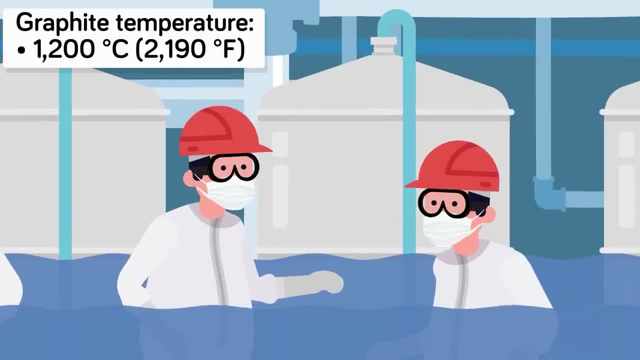 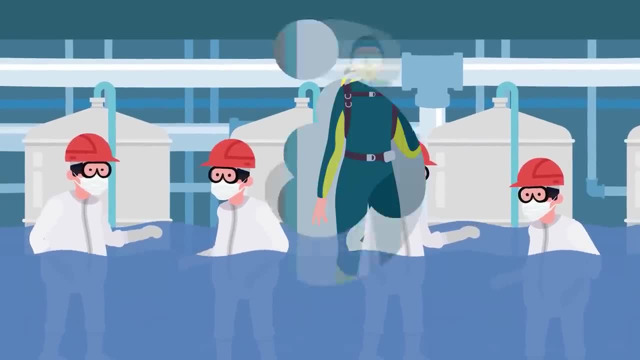 remember, heated to about 1200 degrees Celsius, hits the water, there could be another massive explosion, even bigger than the last one, And that could mean Europe being hit with more radiation. They don't know it yet, but it's highly unlikely this explosion will happen. They think it could. 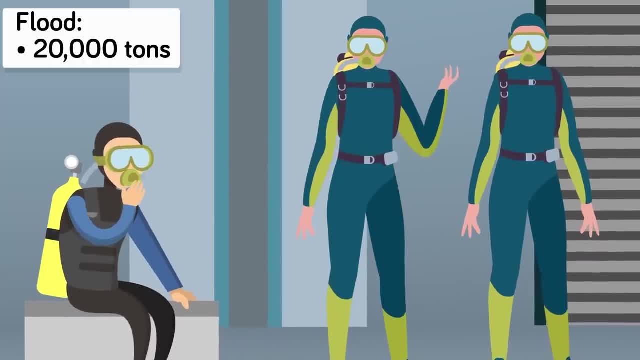 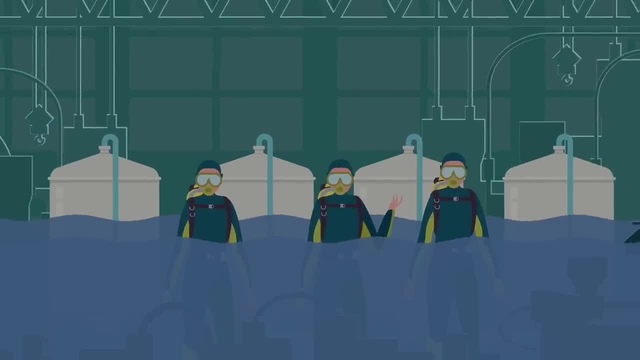 and so tell three men who know the area inside and out that they'll have to drain the 20,000 tons of water through a sluice gate. These men know that there's a good chance they might not make it out, and even if they do, they might not live very long after Hour 58.. The KGB has been. 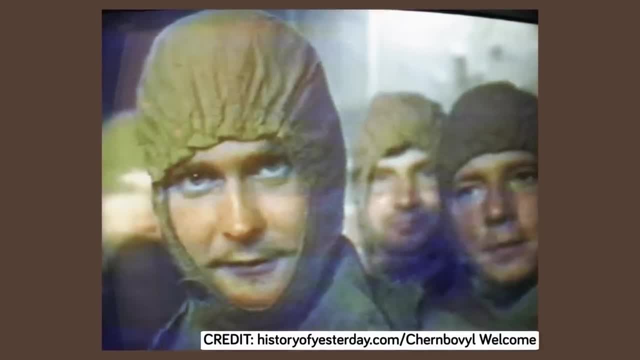 told that the water tanks are empty, which isn't actually the case. To make things worse, they're going to have to drain the 20,000 tons of water through a sluice gate. Hence the name: the Chernobyl Suicide Squad: Alexey Ananyanko, Valery Bezpilov and Boris Baranov. Hour 60.. 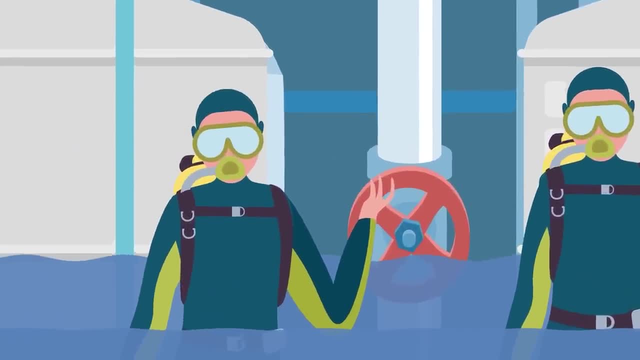 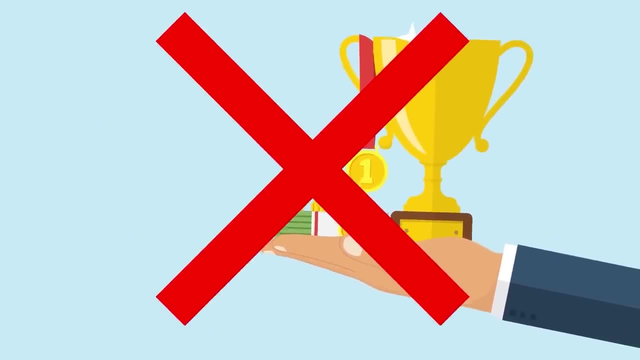 Finding the valves in the dark is like finding a needle in a haystack, but they do it in the end. For them, it's just another day at work. They knew they'd be fired if they didn't do his ask and, unlike what will be said in years to come, they didn't get any reward for their work. 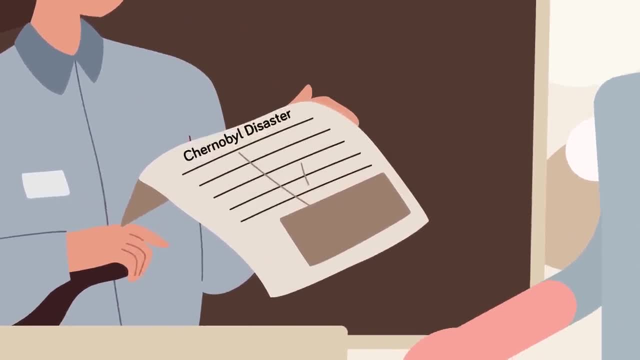 As we've explained, there will be a lot of western misinformation flying about in regard to the Chernobyl disaster. One falsity told time and again is that these three men are the ones who are going to be fired. They're going to be fired. 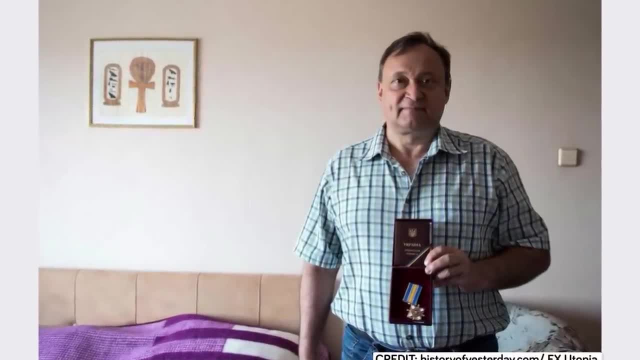 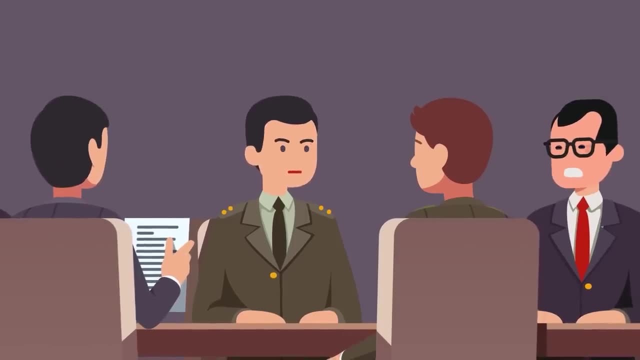 All three men all died shortly after they succeeded in their mission. but they didn't. They lived long, healthy lives after their time in the darkness of Chernobyl Hour 66. The Soviet government is now worried that the Molten Core will burn through the cement and 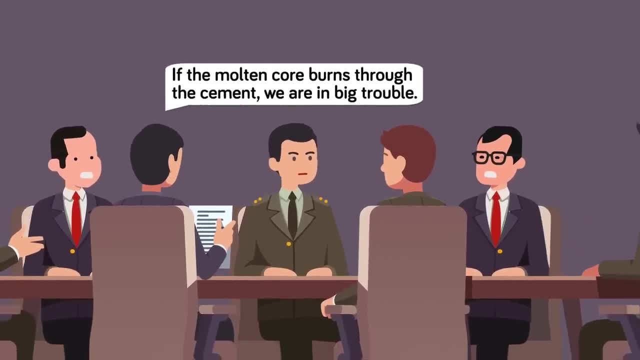 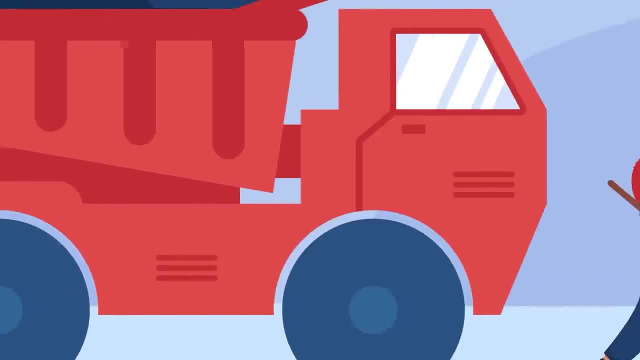 get to the groundwater, thereby contaminating it and spreading radiation to the rest of Ukraine and into Europe, possibly making some places uninhabitable. A mining team is brought in to dig a huge tunnel below the reactor to act as a cooling system, and they're given respirators. 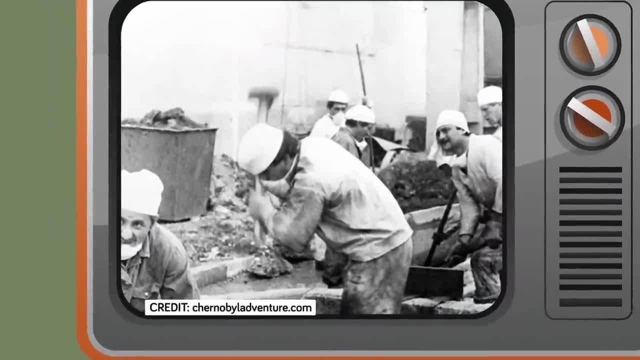 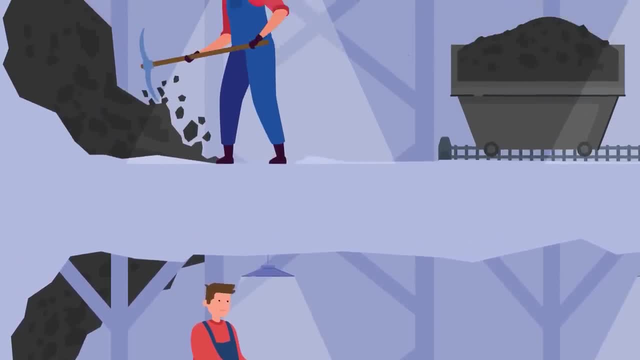 for the work, but it's hard to breathe with them on. It's also very hard to breathe with very hot, But they don't work naked, as will be told in TV in the future. Again, it's a big job and a risky job for the 400 or so miners. The Soviets don't have to be too concerned because 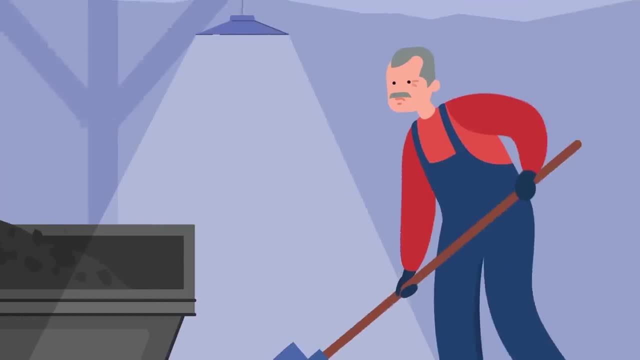 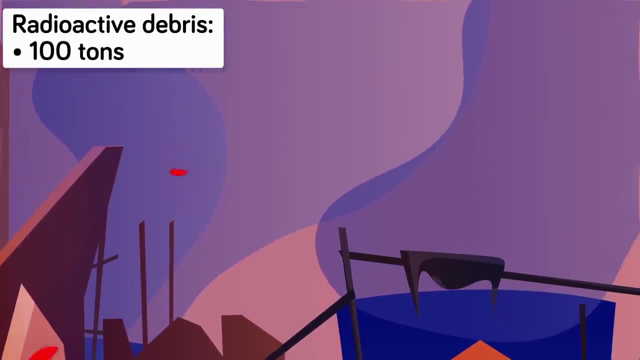 the core won't melt through the concrete. Obviously they don't know that yet and have to take all precautions. Hour 100.. The debris removal starts At first. the 100 tons of radioactive material is said to be so dangerous that the men shouldn't go near it. 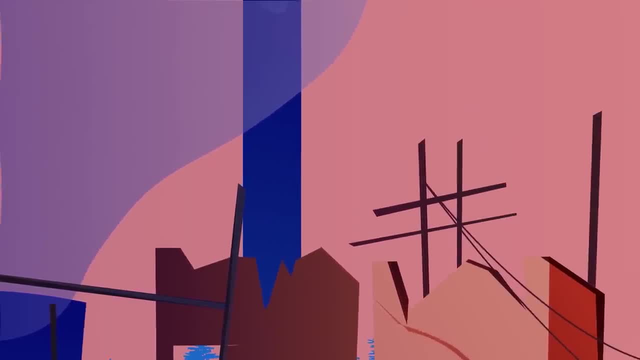 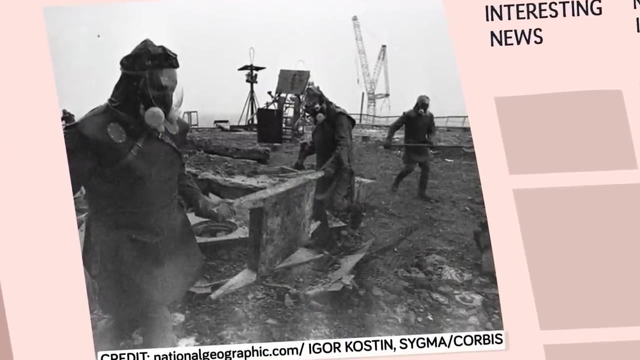 They opt to use robots, but most of the robots break as soon as deployed due to radiation. The liquidators are chosen to do the job- men who are now camping close to the plant. Thousands of them are there and in time, 600,000 or so of them will help with the cleanup. They're given protective clothing. 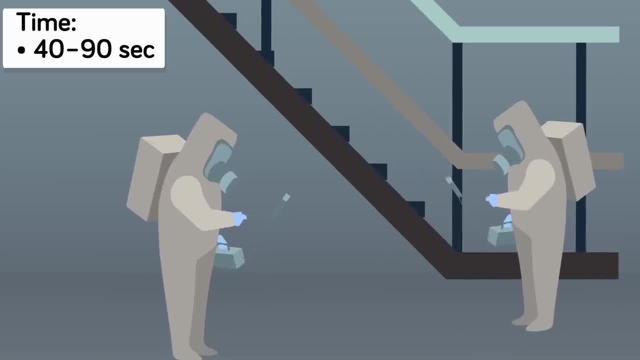 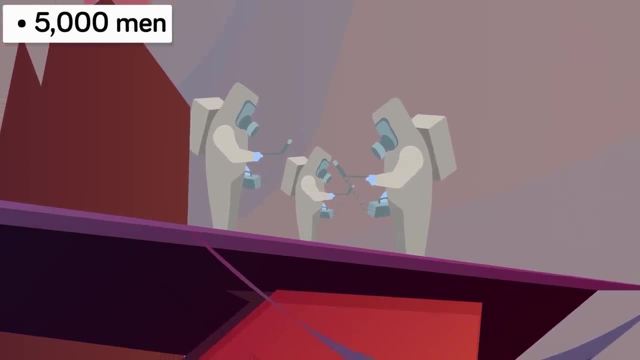 but still told they shouldn't stay on the roof longer than 40 to 90 seconds, since the graphite and other materials up there are about as radioactive as you can get. Of the 5,000 men who do the job, some will go up as many as six times. 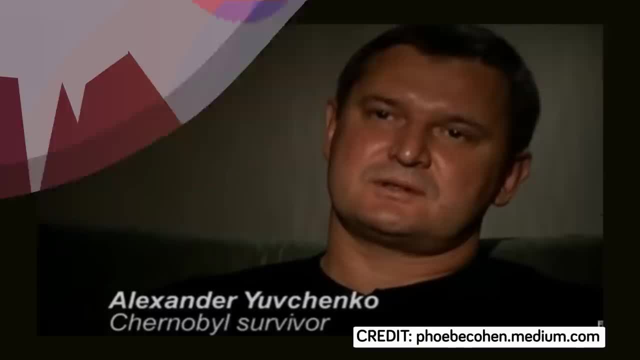 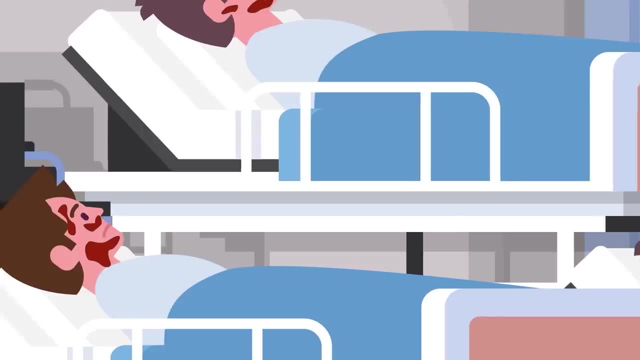 but it's hard to say how many will have health problems because of it. Alexander, as you know, survives. He's flown to Moscow. his hair falls out and he finds it hard to breathe. His eyes, nose and most of his face hurts, but then after a couple days, 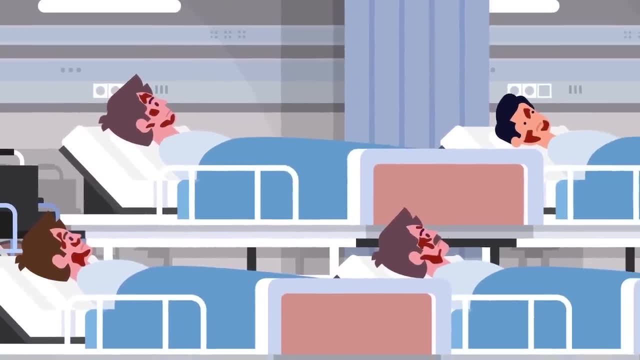 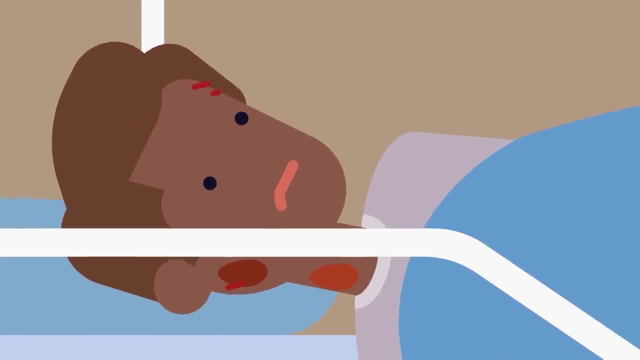 he and the other men all start to feel pretty good. As you already know, this doesn't mean they are good. One day he's in pain again and he pulls back his bedsheets to see massive ulcers and necrotic skin on his shoulder, hip and calf- all the bits exposed when he held the door open. 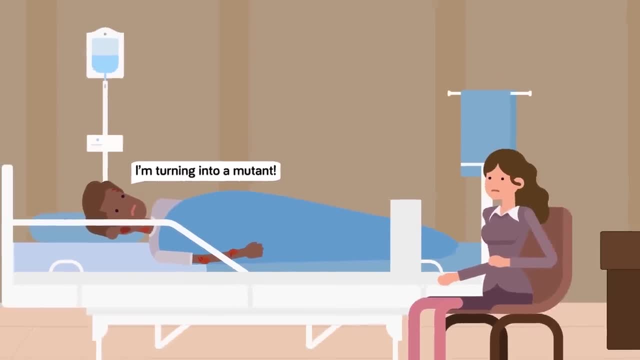 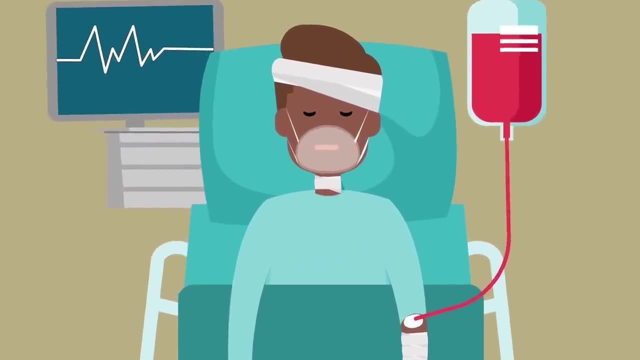 He's turning black and feels like he's a monster, telling himself he looks like some kind of radioactive mutant. Luckily for him, his body accepts the skin grafts, and blood transfusions and bone marrow transplants do the rest. He's in pain and he's in pain and he's in pain. 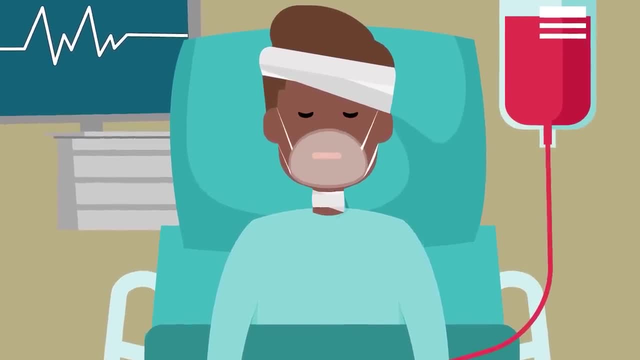 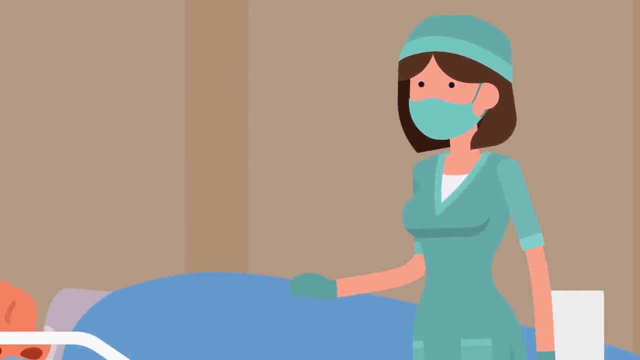 His arm is in really bad shape and will stay in bandages for years In the hospital. every so often someone walks into the room and tells him another of his colleagues is dead. One of them first goes blind and then the infection in his blood finishes him off. For two months, Alexander lies in bed close to death, thinking about how it'll be when it's his turn to die. He will later be awarded medals for his bravery, but once he's better he'll keep his Chernobyl experience mostly to himself For many years to come. 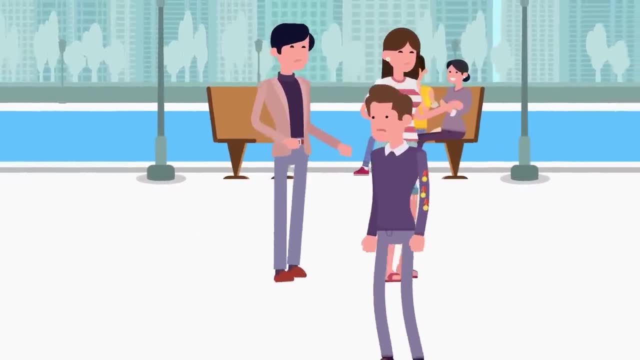 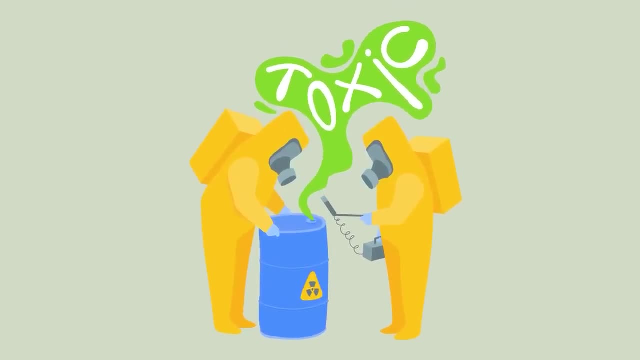 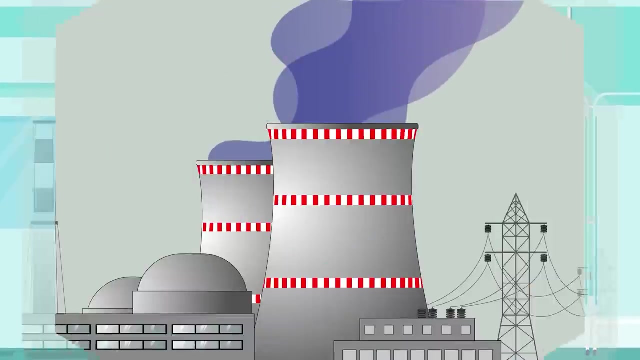 people in this part of the world will cross the street if they see a Chernobyl survivor walking toward them. These people, not educated about radiation, wrongly assume the survivors are contaminated. This fear has devastating consequences. Soon after the disaster, there are 150,000 elective abortions. Chernobyl, in fact, will make much of the world wrongly. 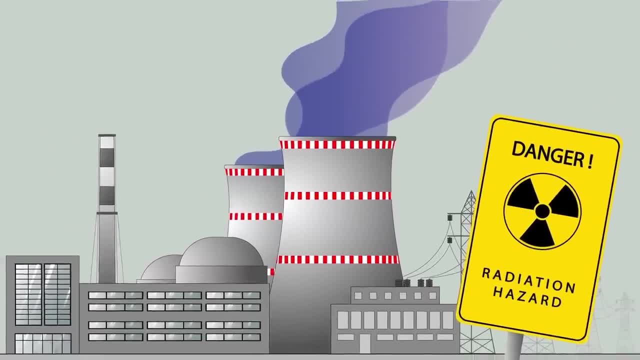 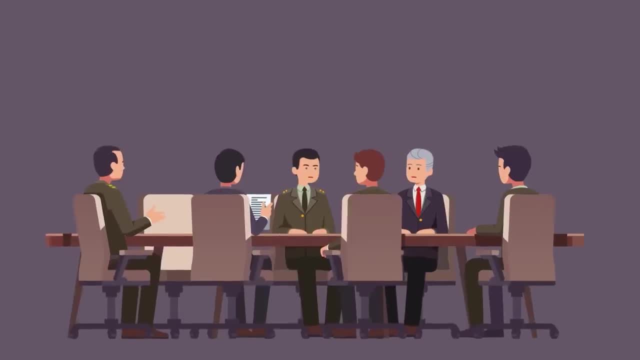 overestimate the dangers of producing nuclear power. This will go on for decades and is still a factor in some people's minds today when they think about nuclear energy. What or who is to blame for the disaster is the question that the Soviets and many other countries will be asking. 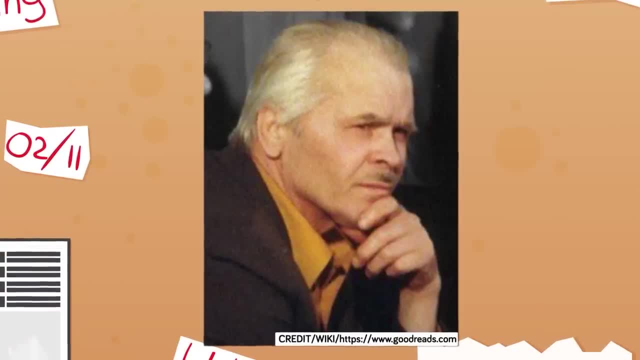 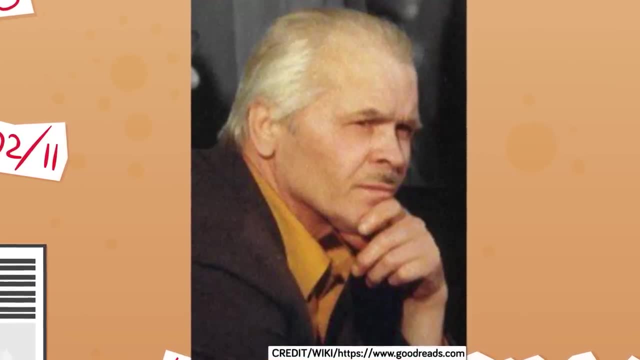 for some time to come. The investigations at the start will mostly blame human error rather than technical error and pick out a few names to shame and send to prison, such as Mr Dyatlov Sure. he messed up a bit, as did others at the plant, but the fault lies. 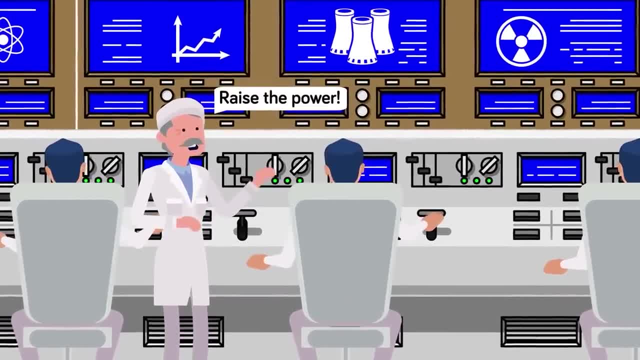 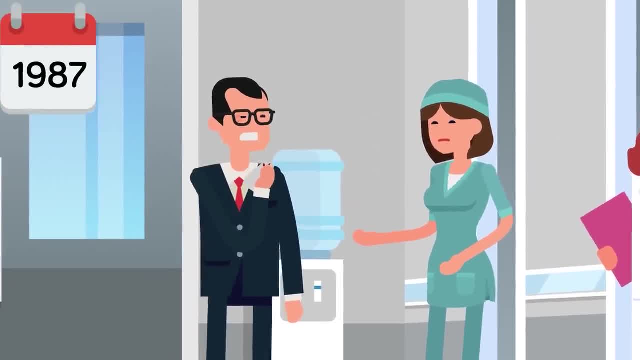 in many people, going right up to the top brass in the communist government. One year later, It's now 1987, and Legasov is very ill from radiation poisoning and is in and out of the hospital all the time. He knows he's going to die, so he records himself. 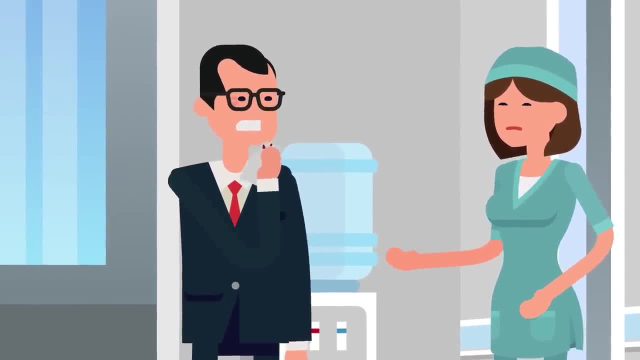 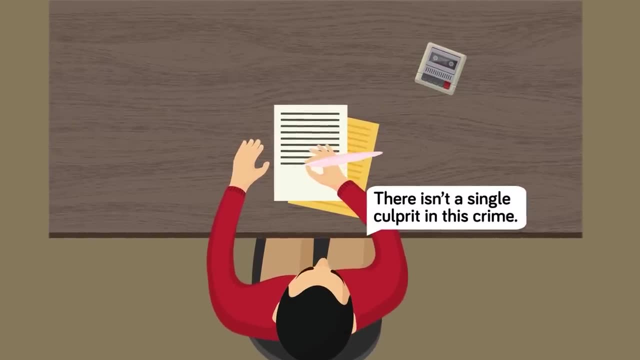 on tape telling the whole truth about how and why this disaster happened. Part of the tape goes: The Chernobyl disaster is an apotheosis, the pinnacle of all the mismanagement that has been carried out for decades in our country. When one looks at the chain of events, why someone 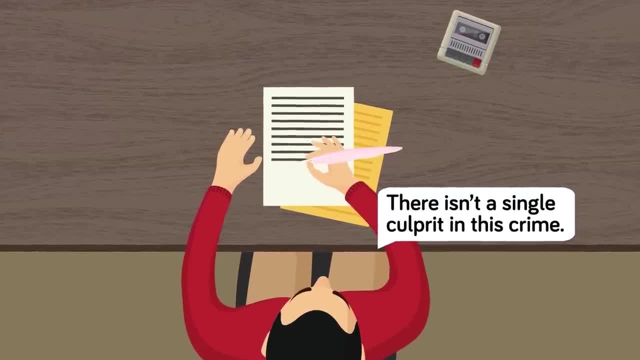 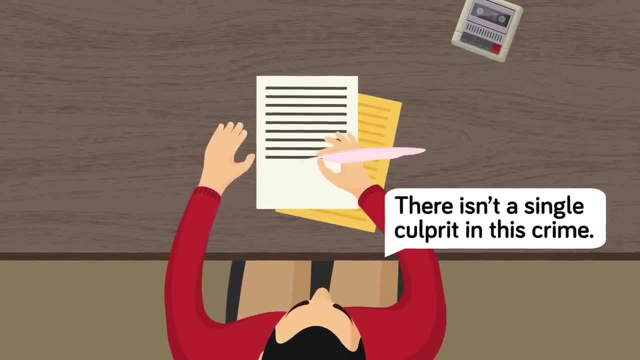 acted in this way and another in that way and so on. it's impossible to point to a single culprit, an initiator of all the unpleasant events that led to the crime, because it's a chain that links to itself. He finishes off by warning that, as he speaks, the Soviet Union does not have a safe 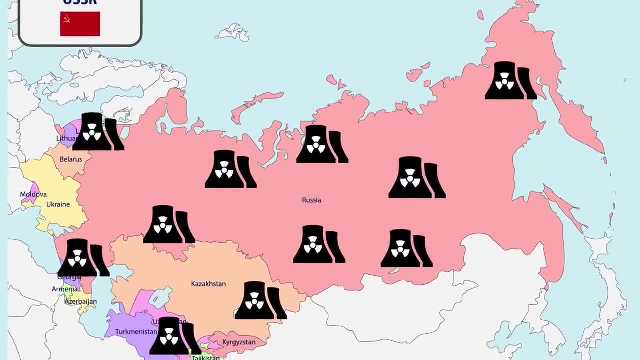 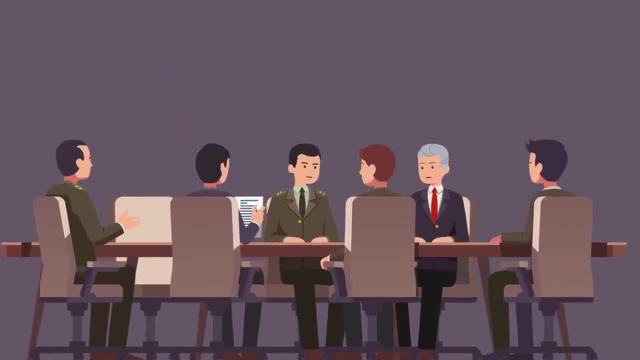 plan, Not because the production of energy is dangerous in itself, but because too many mistakes have been made and too many corners have been cut. He says: when you can't hold the state accountable, then the state is broken. Two years later, In 1988, the day after the second,